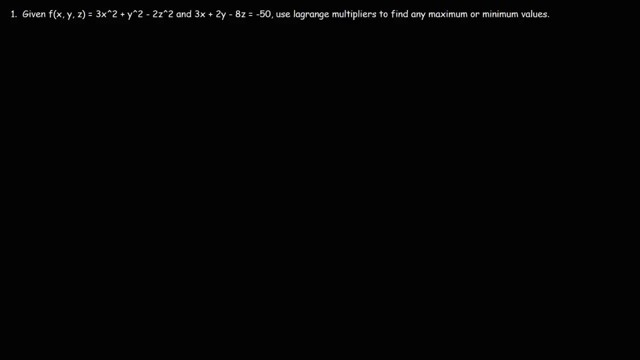 In this video we're going to talk about how to use Lagrange multipliers to find maximum or minimum values. So in a problem like this, we're given a multivariable function- In this case f contains three variables- And we're given a constraint which is g of x, y, z, and that's equal to some constant k. 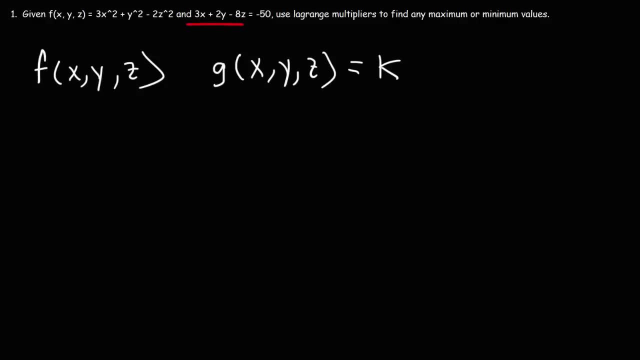 And you can see that g is 3x plus 2y minus 8z. That's the constraint, because it's equal to a constant, in which case, in this case, it's negative 50.. Now what we need to do is we need to write a system of equations to solve for four variables. 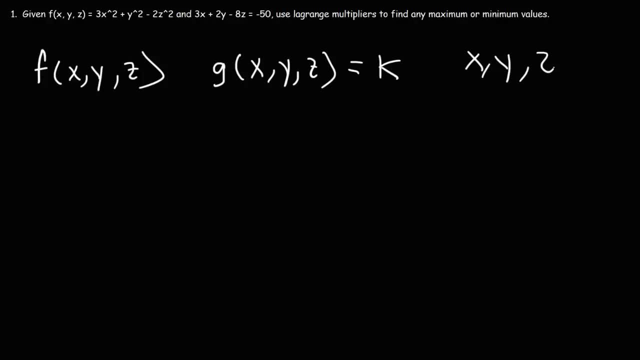 The four variables will be x, y, z and lambda, So the first equation that we need to write will be this one: f- fx is equal to lambda times gx, where fx is the partial derivative of f with respect to x. 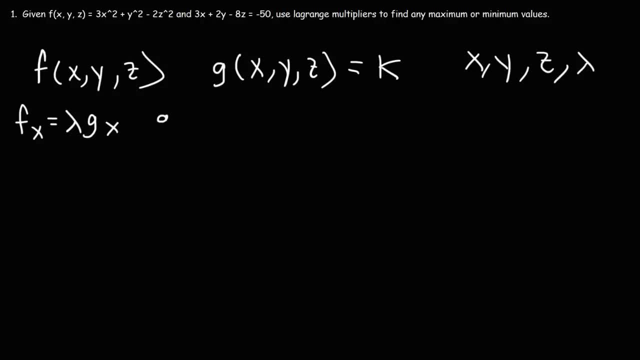 So that's the first equation that we need to write. The second one is going to be the partial derivative of f with respect to y, and that's going to equal lambda times gy. The next one is going to be: fz is equal to lambda gz. 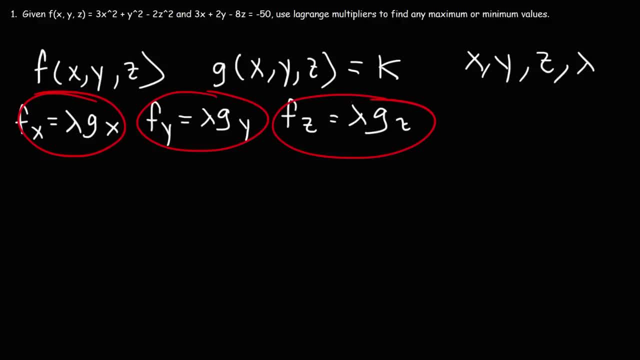 So here we have 1,, 2,, 3, 4 equations. So we have a system of four equations which we need in order to solve for four variables. So that's what we're doing here in this example problem. So let's start with the first equation. 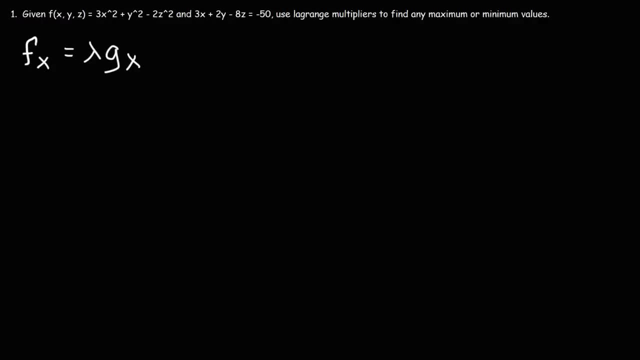 fx is equal to lambda gx. So the partial derivative of this expression with respect to x- y squared and negative 2z squared will go to zero, because we're going to treat them as constants. The derivative of 3x squared, that's going to be 3 times 2x. 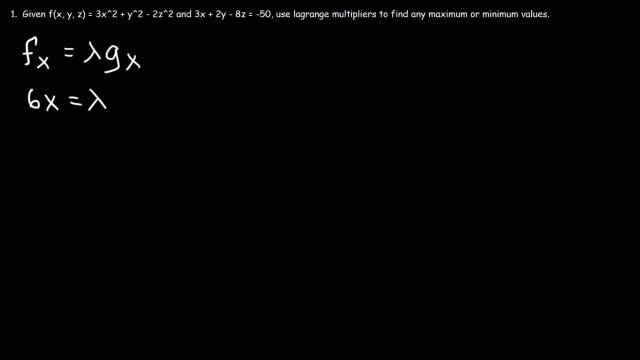 which is 6x, And that's equal to lambda. And then we need to differentiate this expression with respect to x. 2y, negative 8z and negative 50 are constants, So when we differentiate them with respect to x, they will become zero. 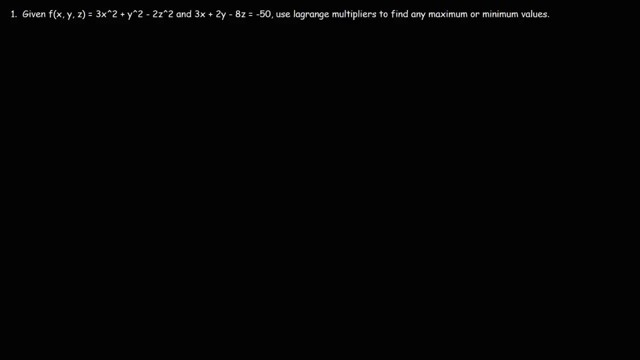 In this video we're going to talk about how to use Lagrange multipliers to find maximum or minimum values. So in a problem like this, we're given a multivariable function- In this case f contains three variables- And we're given a constraint which is g of x, y, z, and that's equal to some constant k. 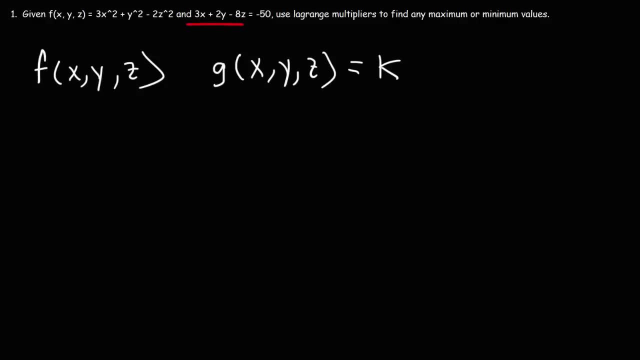 And you can see that g is 3x plus 2y minus 8z. That's the constraint, because it's equal to a constant, in which case, in this case, it's negative 50.. Now what we need to do is we need to write a system of equations to solve for four variables. 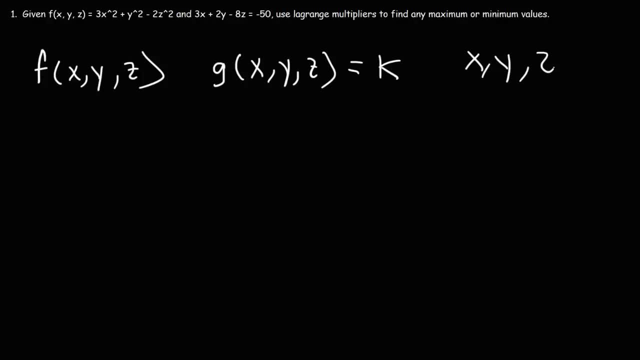 The four variables will be x, y, z and lambda, So the first equation that we need to write will be this one: f- fx is equal to lambda times gx, where fx is the partial derivative of f with respect to x. 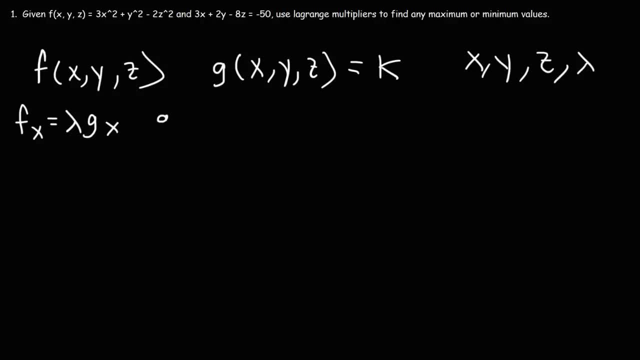 So that's the first equation that we need to write. The second one is going to be the partial derivative of f with respect to y, and that's going to equal lambda times gy. The next one is going to be: fz is equal to lambda gz. 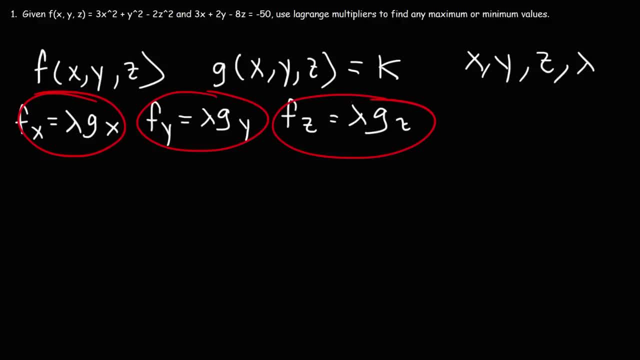 So here we have 1,, 2,, 3, 4 equations. So we have a system of four equations which we need in order to solve for four variables. So that's what we're doing here in this example problem. So let's start with the first equation. 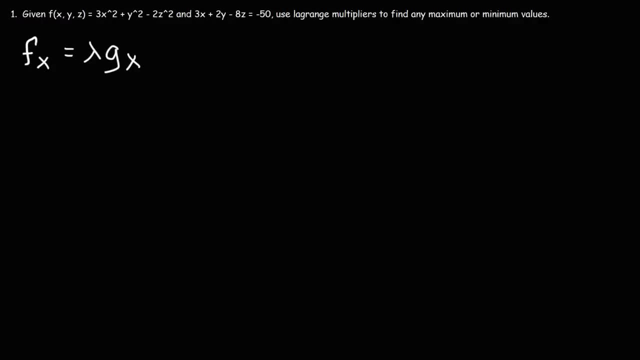 fx is equal to lambda gx. So the partial derivative of this expression with respect to x- y squared and negative 2z squared will go to zero, because we're going to treat them as constants. The derivative of 3x squared, that's going to be 3 times 2x. 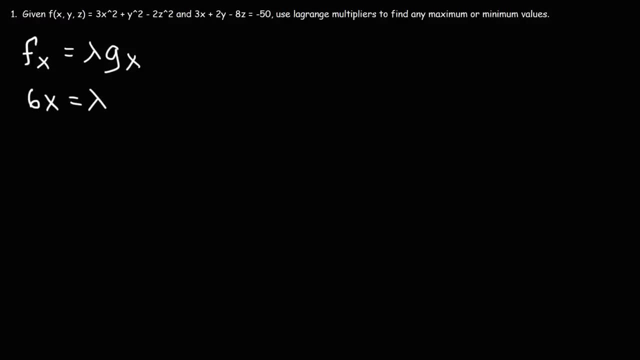 which is 6x, And that's equal to lambda. And then we need to differentiate this expression with respect to x. 2y, negative 8z and negative 50 are constants, So when we differentiate them with respect to x, they will become zero. 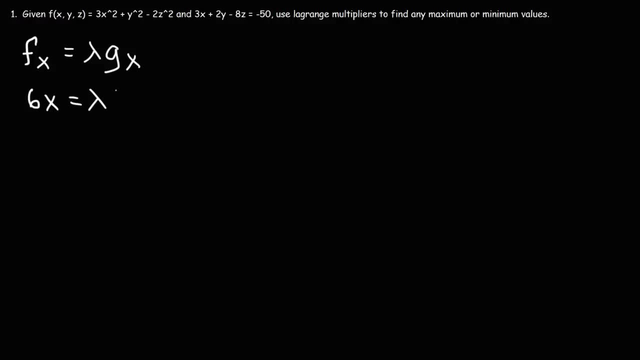 3x will become 3.. So that's gy. So now what we're going to do here is we're going to solve for x, So let's divide both sides by 6. We're going to get x in terms of lambda. 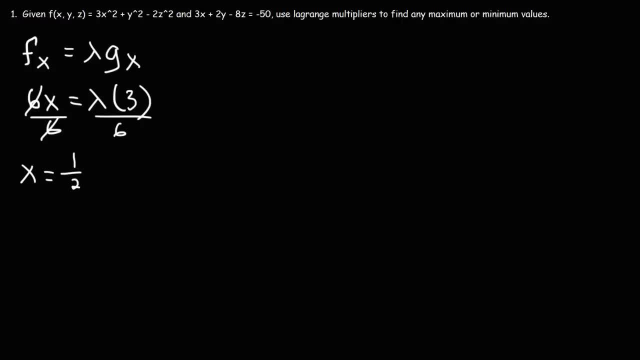 3 over 6 is 1 half, So x is 1 half lambda. Now let's move on to our next equation. fy is equal to lambda gy, So the derivative of f with respect to y. we just need to differentiate it. 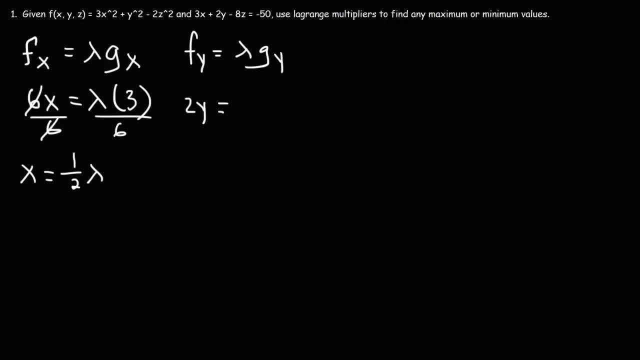 We're going to differentiate y squared, which becomes 2y, The derivative of g with respect to y, we just need to find the derivative of 2y, which is 2.. So, isolate in y, we're going to divide both sides by 2.. 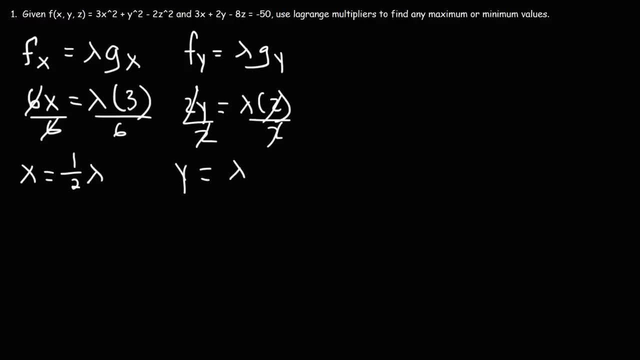 And so we have the expression that y is equal to lambda. Now for the next one we have. fz is equal to lambda gz. The derivative of negative 2z squared, that's going to be negative 4z, And the derivative of negative 8z is just negative 8.. 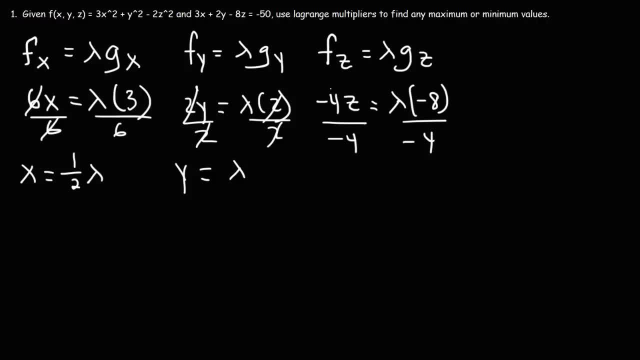 So now let's divide both sides by negative 4 to get z. So negative 8 divided by negative 4, that's positive 2.. So z is 2 times lambda. So now we're going to get rid of this, And what we're going to do now is we are going to replace x, y and z. 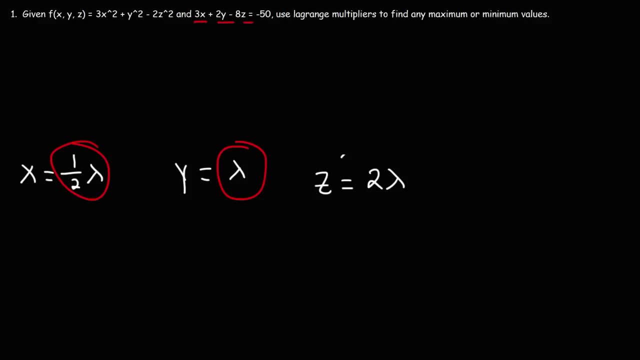 in our constraint with what we see here. So we can get one equation with one variable, And that equation will be in terms of lambda. So we have 3x, but we're going to replace x with 1 half lambda And then plus 2y or 2 times lambda. 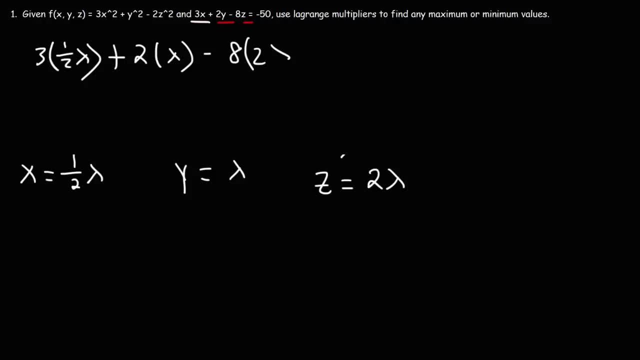 Minus 8.. And then z is 2 lambda And all of that is going to equal negative 50. So we have 3 over 2 lambda plus. So this is 2 lambda minus 16 lambda. That's going to be negative 14 lambda. 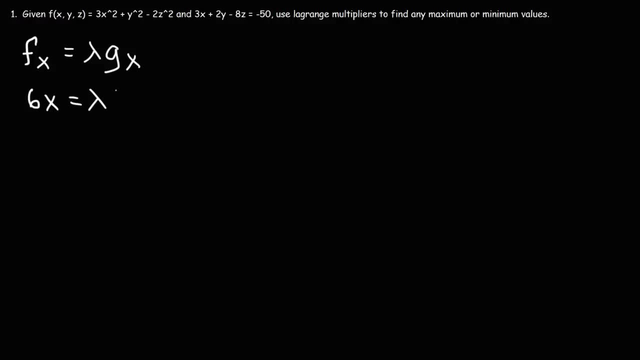 3x will become 3.. So that's gy. So now what we're going to do here is we're going to solve for x, So let's divide both sides by 6. We're going to get x in terms of lambda. 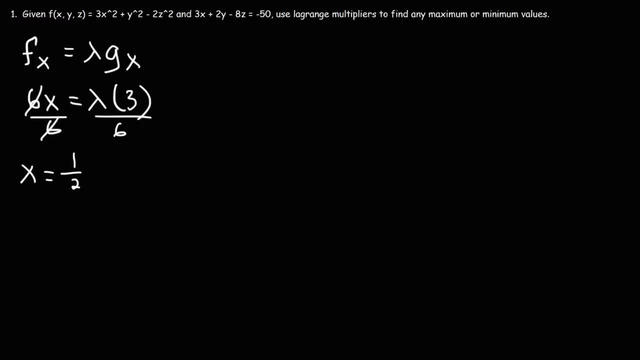 3 over 6 is 1 half, So x is 1 half lambda. Now let's move on to our next equation. fy is equal to lambda gy, So the derivative of f with respect to y. we just need to differentiate. 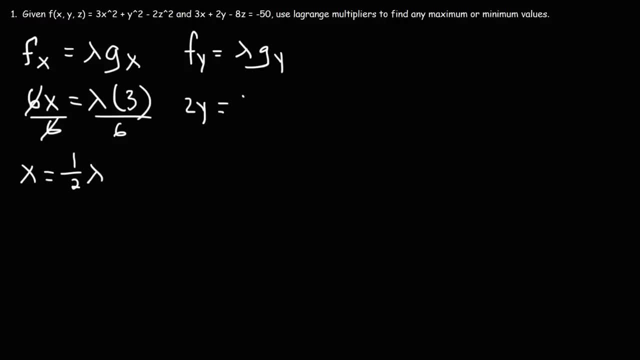 y squared, which becomes 2y, The derivative of g with respect to y. we just need to find the derivative of 2y, which is 2.. So, isolate in y, we're going to divide both sides by 2.. 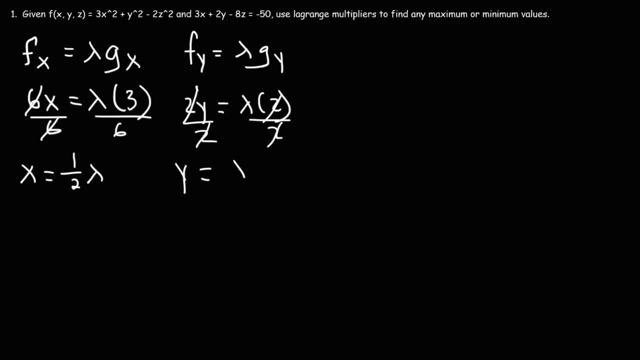 And so we have the expression that y is equal to lambda. Now for the next one we have. fz is equal to lambda gz. The derivative of negative 2z squared, that's going to be negative 4z, And the derivative of negative 8z is just negative 8.. 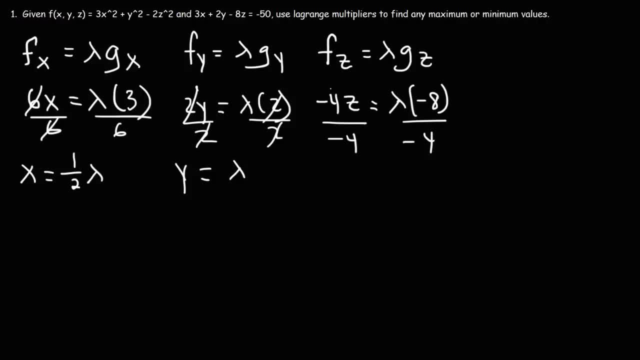 So now let's divide both sides by negative 4 to get z. So negative 8 divided by negative 4, that's positive 2.. So z is 2 times lambda. So now we're going to get rid of this, And what we're going to do now is we are going to replace x, y and z. 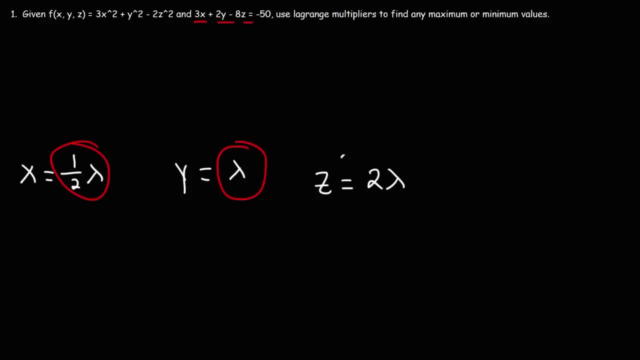 in our constraint with what we see here. So we can get one equation with one variable, And that equation will be in terms of lambda. So we have 3x, but we're going to replace x with 1 half lambda And then plus 2y or 2 times lambda. 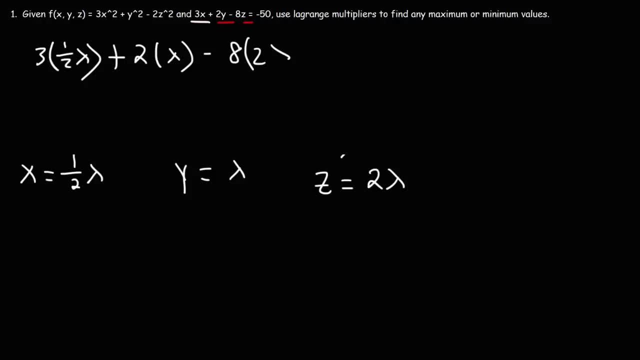 Minus 8.. And then z is 2 lambda And all of that is going to equal negative 50. So we have 3 over 2 lambda plus. So this is 2 lambda minus 16 lambda. That's going to be negative 14 lambda. 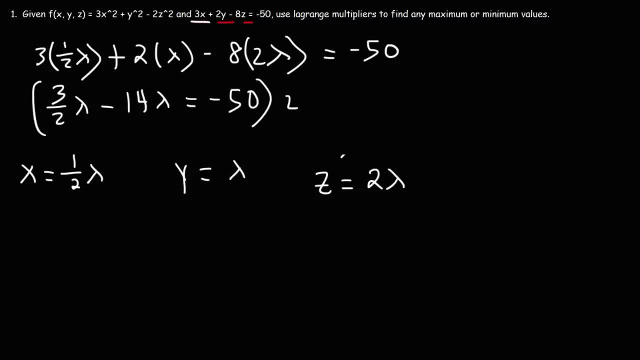 Now to get rid of the fraction, let's multiply everything by 2.. So 3 over 2 times 2.. That's just going to be 3.. So we're going to have 3 lambda And then 2 times negative 14.. 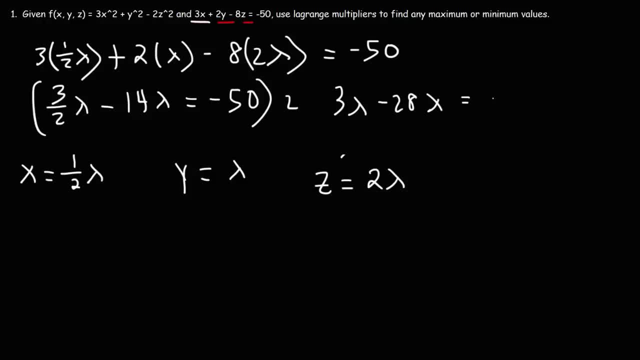 That's negative 28.. And this is going to be negative 50 times 2,, which is negative 100.. So now we can combine those two: 3 minus 28 is negative 25.. Dividing both sides by negative 25.. 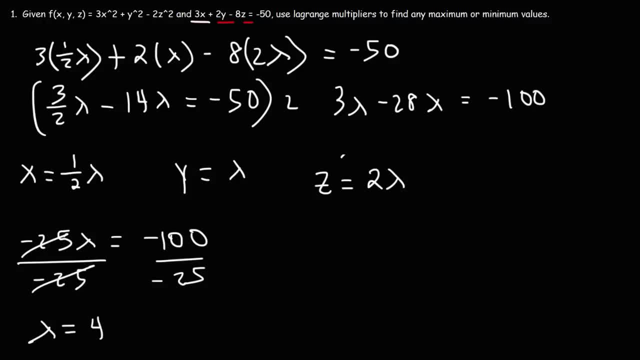 We have lambda, It's going to be 4.. So now that we have lambda, We can plug it back in to get our values for x, y and z. So, starting with x, x is 1, half of lambda, 1 half of 4 is 2.. 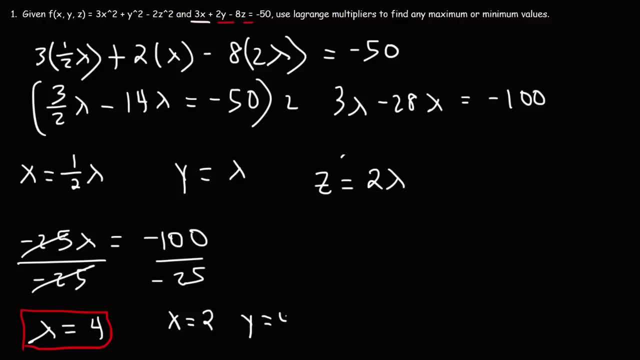 y is equal to lambda, Lambda is 4,, so y is 4.. And z is 2 times lambda, Or 2 times 4,, which is 8.. So we have the point 2,, 4, and 8.. 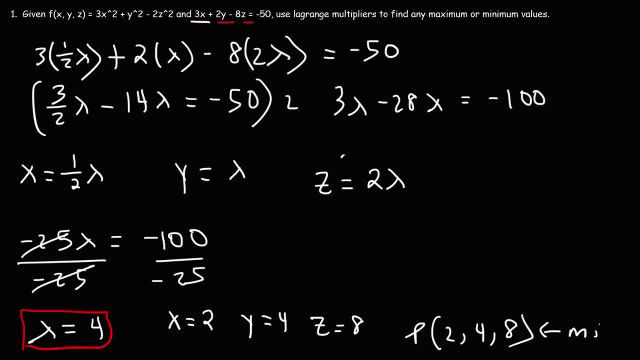 It turns out that we have 2 times lambda And it turns out that this point is a minimum. And the way you can check if it's a minimum or not Is you can plug in another point and see if it's going to be higher or lower than f. 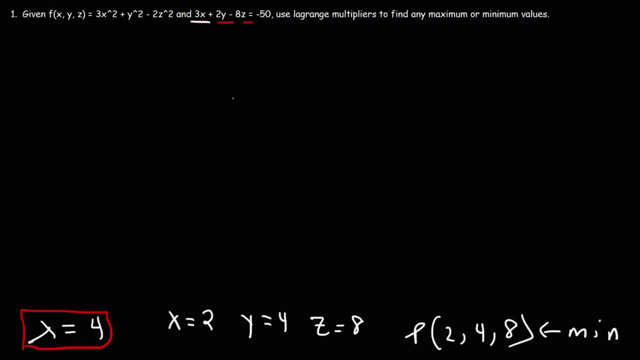 Whatever point you choose, you need to make sure that it still fits in the constraint. So you can't just change 2 into 3, because it's not going to equal negative 50. So let's plug in the point that we have into the function. 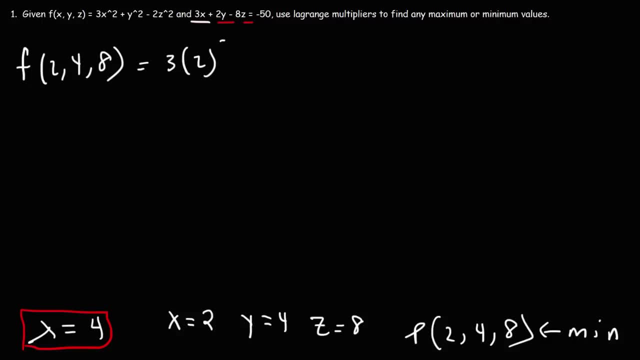 So this is going to be 3 times 2 squared Plus 4 squared, minus 2 times 8 squared. So 2 squared is 4 times 3, that's 12.. 4 squared is 16.. 8 squared is 64 times 2, that's 128.. 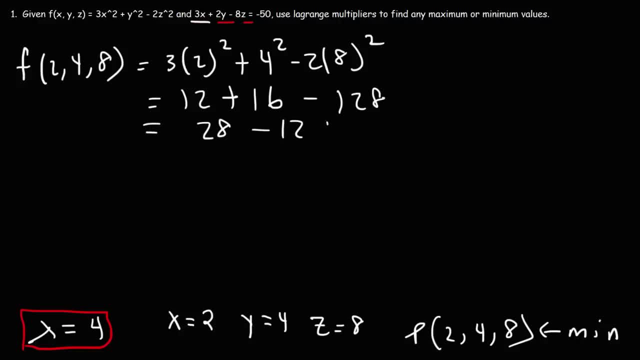 12 and 16 is 28.. 28 minus 128 is negative 100. So that is the minimum. That is the minimum value of the function. Now let's say if we were to try another point like f of 4 comma negative 3 comma 7.. 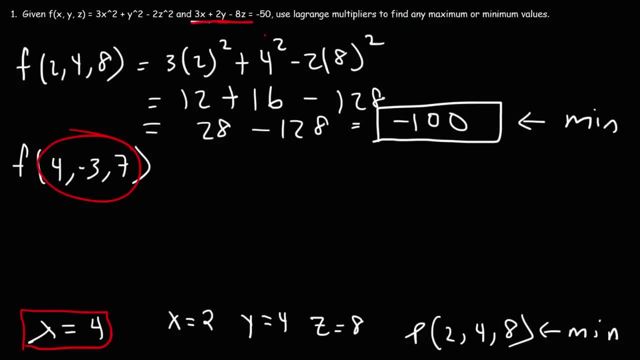 If you plug in those values into this expression, you're going to get negative 50. This gives you a higher value of negative 41. Negative 41 is higher than negative 100. And if you try another point like 0,, 11,, 9.. 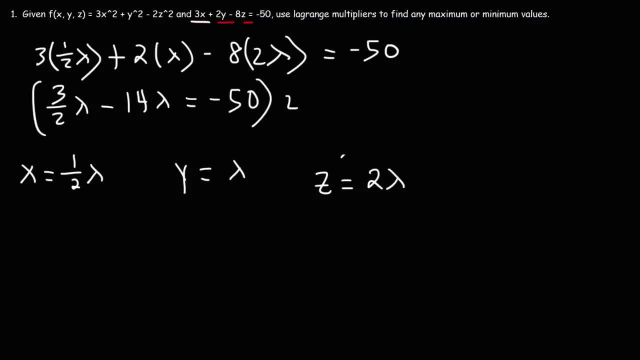 Now to get rid of the fraction, let's multiply everything by 2.. So 3 over 2 times 2.. That's just going to be 3.. So we're going to have 3 lambda And then 2 times negative 14.. 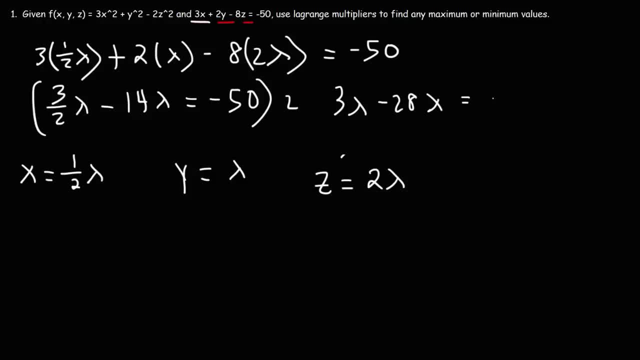 That's negative 28.. And this is going to be negative 50 times 2,, which is negative 100.. So now we can combine those two: 3 minus 28 is negative 25.. Dividing both sides by negative 25.. 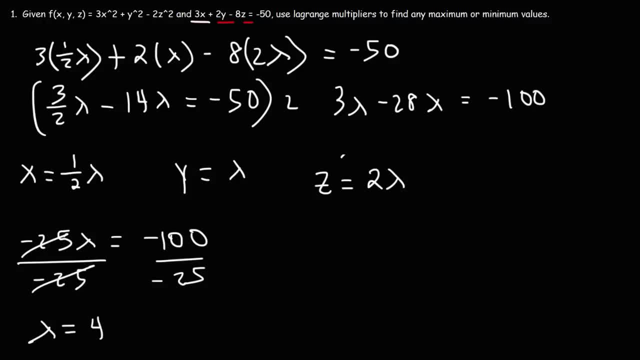 We have lambda, It's going to be 4.. So now that we have lambda, We can plug it back in to get our values for x, y and z. So, starting with x, x is 1, half of lambda, 1 half of 4 is 2.. 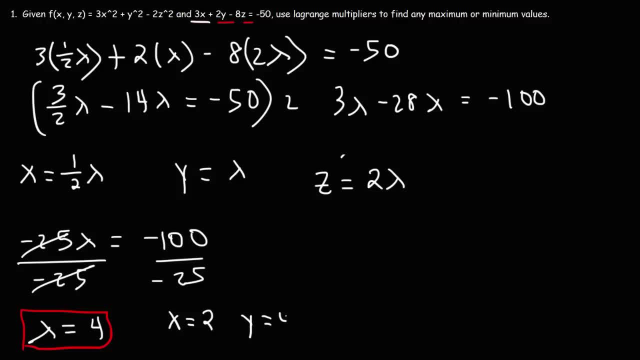 y is equal to lambda, Lambda is 4,, so y is 4.. And z is 2 times lambda, Or 2 times 4,, which is 8.. So we have the point 2,, 4, and 8.. 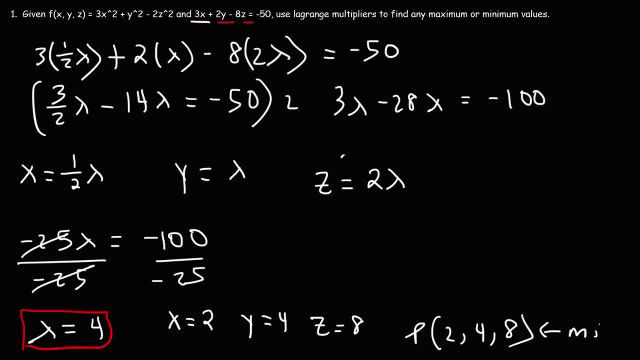 It turns out that we have 2 times lambda. It turns out that this point is a minimum, And the way you can check if it's a minimum or not is you can plug in another point and see if it's going to be higher or lower than f. 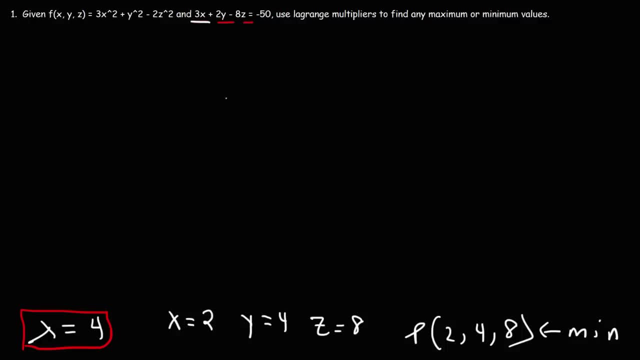 Whatever point you choose, you need to make sure that it still fits in the constraint. So you can't just change 2 into 3, because it's not going to equal negative 50. So let's plug in the point that we have into the function. 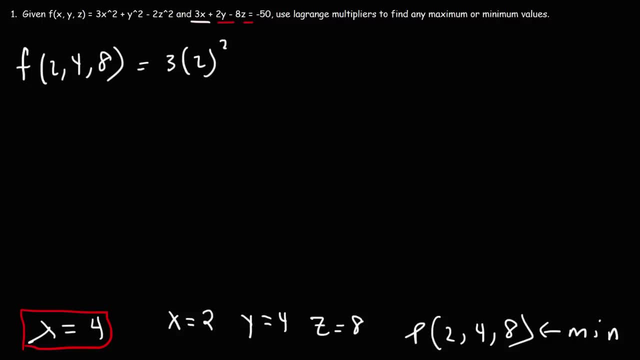 So this is going to be 3 times 2 squared plus 4 squared, minus 2 times 8 squared. So 2 squared is 4 times 3, that's 12.. 4 squared is 16.. 8 squared is 64 times 2, that's 128.. 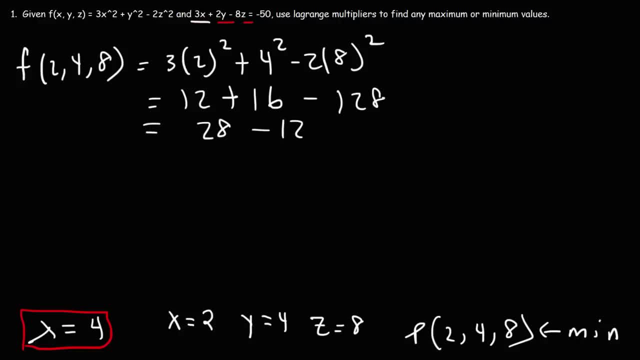 12 and 16 is 28.. 28 minus 128 is negative 100. So that is the minimum value of the function. Now let's say if we were to try another point like f of 4 comma negative 3 comma 7.. 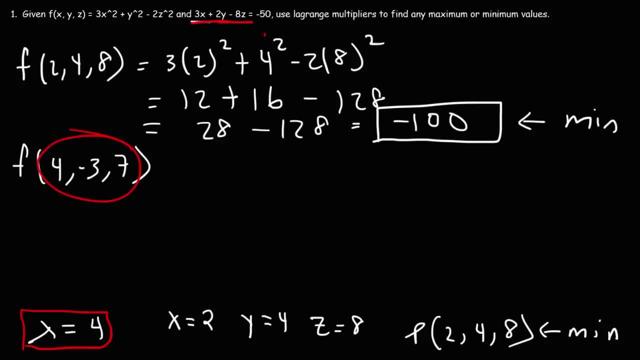 If you plug in those values into this expression, you're going to get negative 50. This gives you a higher value of negative 41. Negative 41 is higher than negative 100.. And if you try another point like 0,, 11,, 9,, 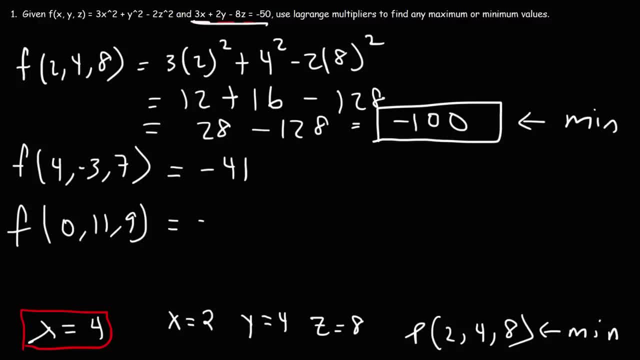 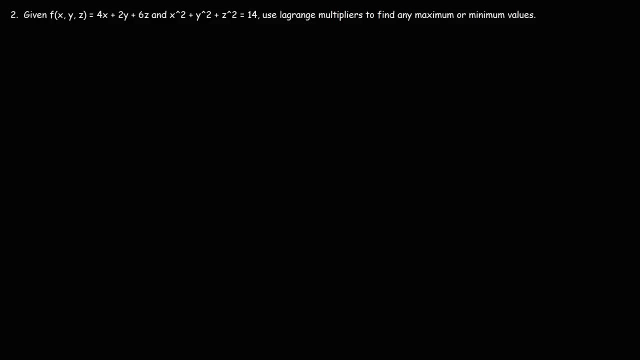 which also fits the constraint. this will give you negative 41 as well, And so this is our minimum value, and it's located at the point 2, comma 4, comma 8.. Now let's work on another problem. Feel free to pause the video and work on this example if you want to. 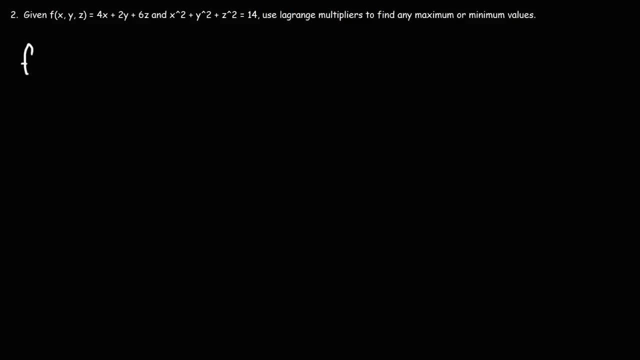 So, just like before, we're going to find fx and set it equal to lambda times gx. So we have our function f and this is g because, as we can see, it's equal to k. k is 14.. So the derivative of 4x is going to be 4.. 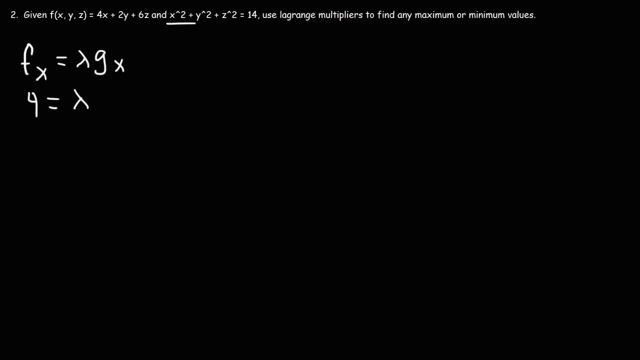 And the partial derivative of g with respect to x is going to be the derivative of x squared, which is 2x. Now, like before, we're going to isolate, So let's divide both sides by 2 lambda. So we have 4 divided by 2 lambda. 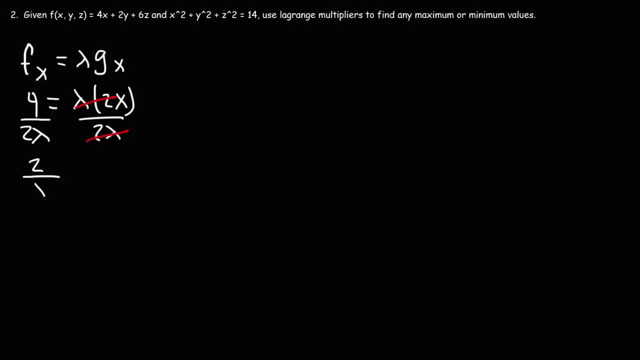 4 divided by 2 is 2.. So x is equal to 2 over lambda. Now let's move on to our next equation. fy is equal to lambda times gy. The derivative of 2y Is 2.. The derivative of y squared is 2y. 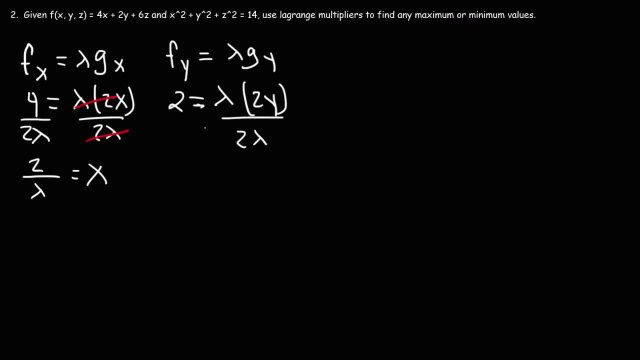 So we're going to isolate y by dividing both sides by 2 times lambda. So 2 divided by 2 is 1.. So this is going to give us 1 over lambda, which is equal to y. Now let's move on to the next one. 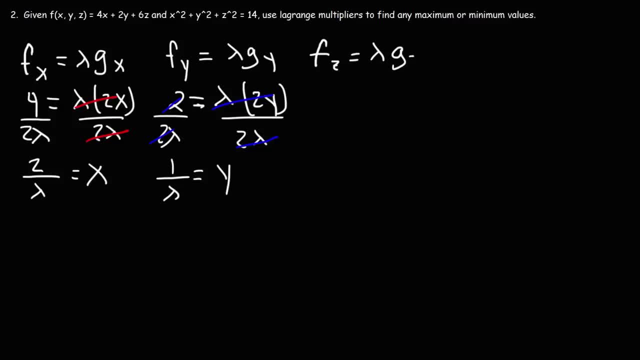 fz is equal to 1 over lambda. So this is going to give us 1 over lambda, which is equal to y. Now let's move on to the next one. fz is equal to lambda gz. The derivative of 6z is going to be 6.. 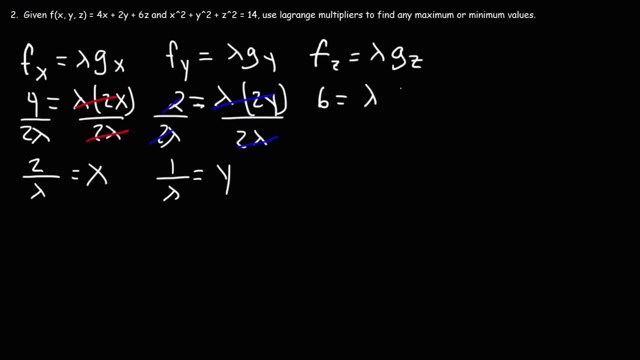 And the derivative of z squared is 2 times z. So divide both sides by 2 lambda. We're going to get z is equal to 6. divided by 2 is 3.. So this is going to be 3 over lambda. 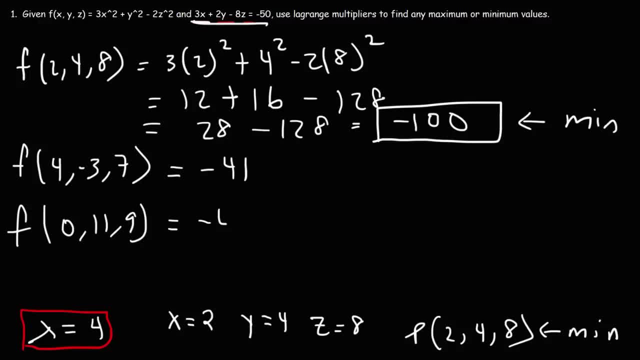 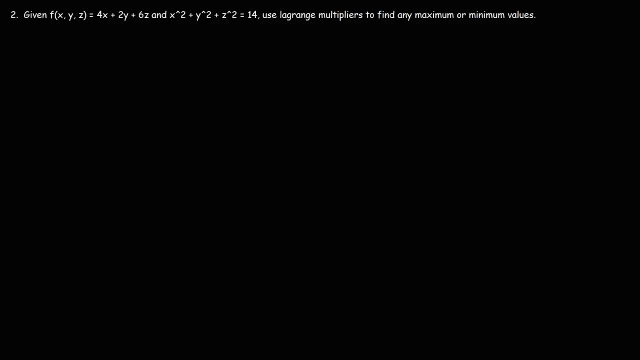 Which also fits the constraint. This will give you negative 41 as well, And so this is our minimum value, and it's located at the point 2, comma 4, comma 8.. Now let's work on another problem. Feel free to pause the video and work on this example if you want to. 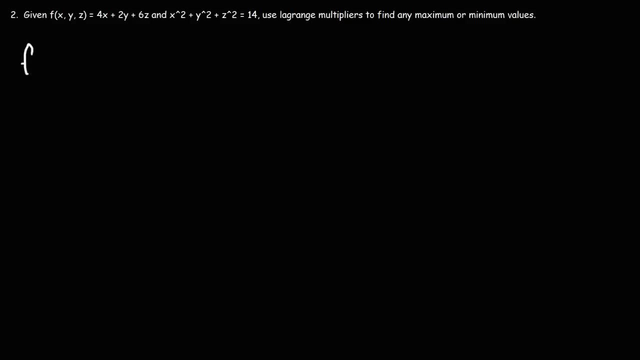 So, just like before, we're going to find fx and set it equal to lambda times gx. So we have our function fx And this is g because, as we can see, it's equal to k. k is 14.. So the derivative of 4x is going to be 4.. 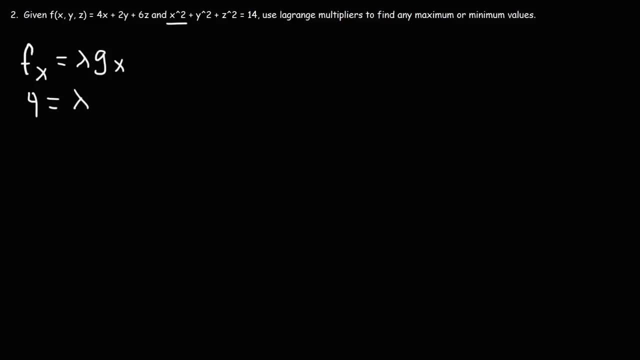 And the partial derivative of g with respect to x is going to be the derivative of x squared, which is 2x. Now, like before, we're going to isolate x. So let's divide both sides by 2 lambda. So we have 4 divided by 2 lambda. 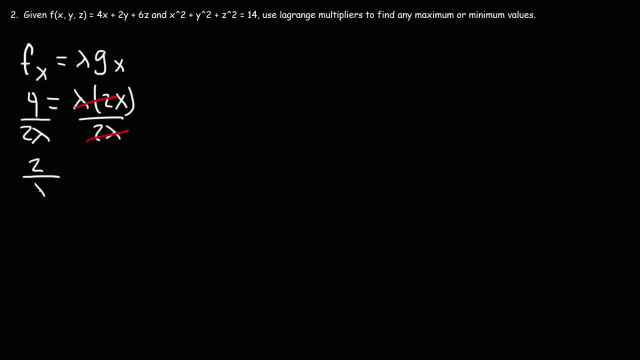 4 divided by 2 is 2.. So x is equal to 2 over lambda. Now let's move on to our next equation. fy is equal to lambda times gy. The derivative of 2y is 2.. The derivative of y squared is 2y. 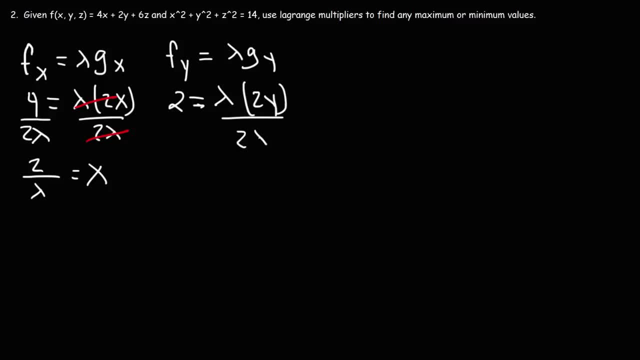 So we're going to isolate y by dividing both sides by 2 times lambda. So 2 divided by 2 is 1.. So this is going to give us 1 over lambda, which is equal to y. Now let's move on to the next one. 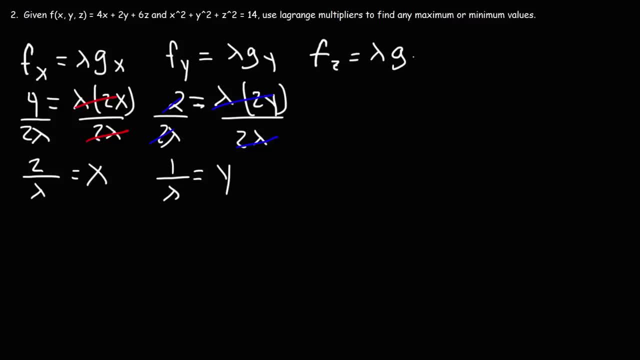 fz is equal to lambda. fz is equal to lambda times gz. The derivative of 6z is going to be 6.. And the derivative of z squared is 2 times z. So divide both sides by 2 lambda We're going to get. z is equal to 6. divided by 2 is 3.. 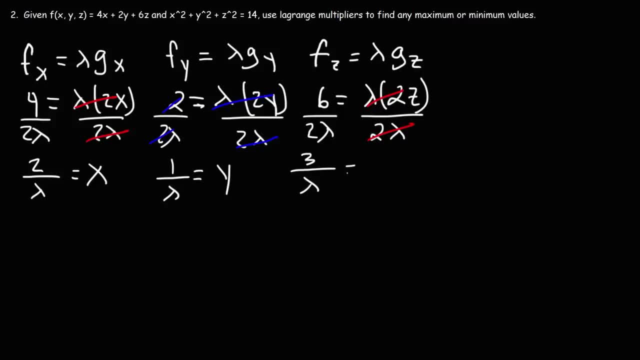 So this is going to be 3 over lambda. So now we have x, y and z in terms of y. So now we have x, y and z in terms of y. So now we have x, y and z in terms of y. 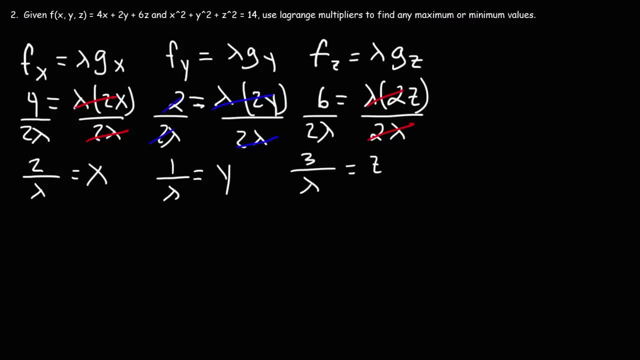 So now we have x, y and z in terms of lambda. So we're going to plug everything into our constraint. We're going to replace x with 2 over lambda, y with 1 over lambda and z with 3 over lambda. 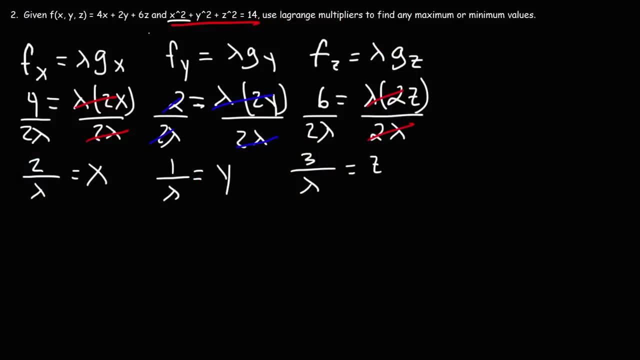 So let's go ahead and do that. So, instead of x squared, it's going to be 2 over lambda squared, And then, instead of y squared, it's going to be 1 over lambda squared, And then plus z squared, which is 3 over lambda squared. 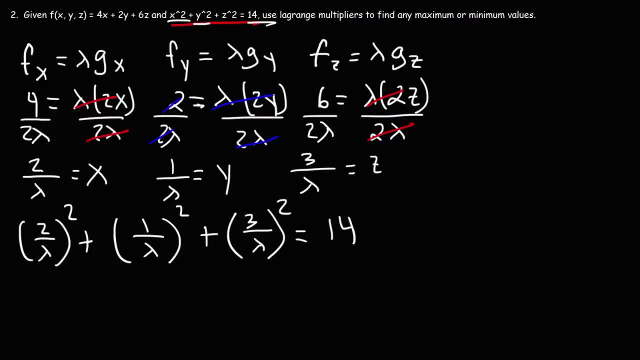 And that's equal to k, which is 14.. So 2 squared is 4.. So this is going to be 4 over lambda squared, And then, plus 1 over lambda squared, 3 squared is 9.. And that's equal to 14.. 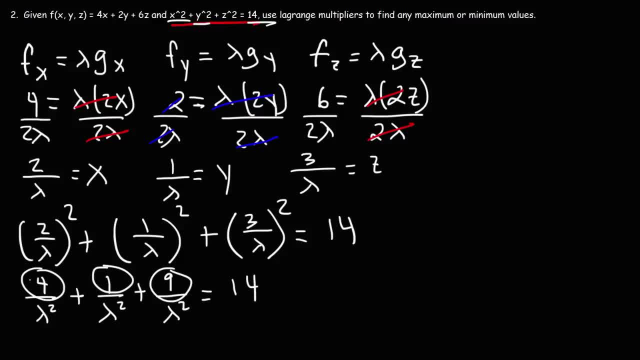 So, adding the numerators, we have 1 plus 9, which is 10, plus 4,, that's 14.. So 14 over lambda squared is equal to 14. And we can put this over 1 and cross multiply. 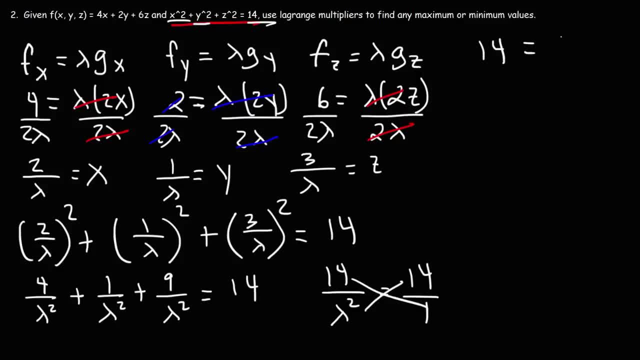 So 14 times 1 is 14.. And then that's equal to 14 lambda squared. So dividing both sides by 14, we see that lambda squared is equal to 1.. And then if we take the square root of both sides, lambda is going to be plus or minus 1.. 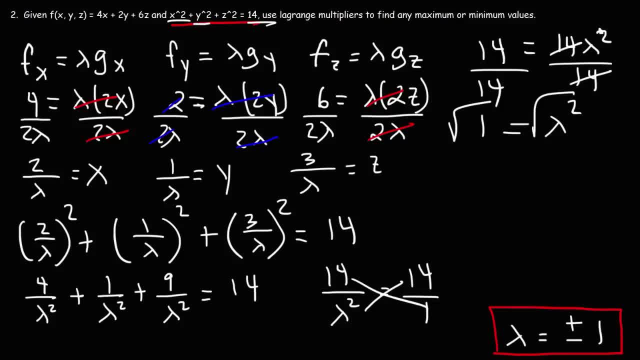 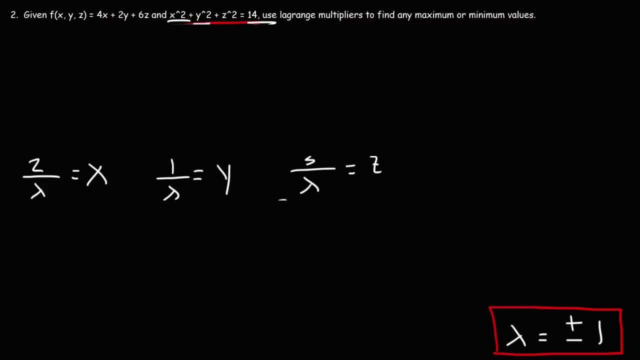 So we have two answers for lambda in this example. So let's talk about what we're going to do with that, But first let's free up some space. Now, if lambda is equal to 1, x is going to be 2 over lambda squared. 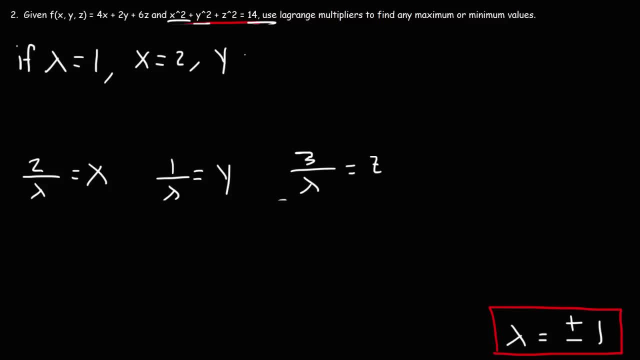 2 over lambda, or 2 divided by 1, which is 2.. y is 1 over lambda, 1 divided by 1, that's 1., And z is 3 over lambda, which will be 3.. 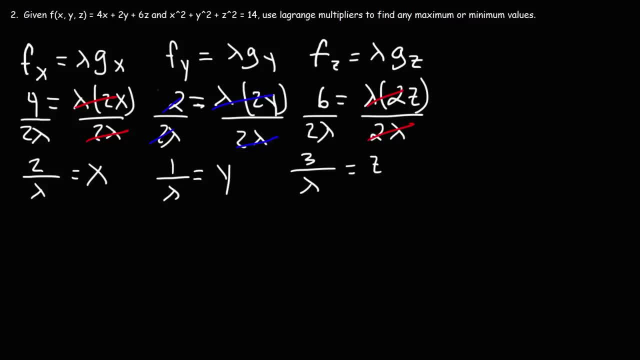 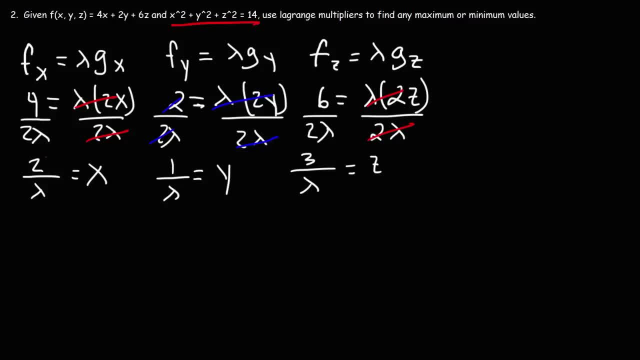 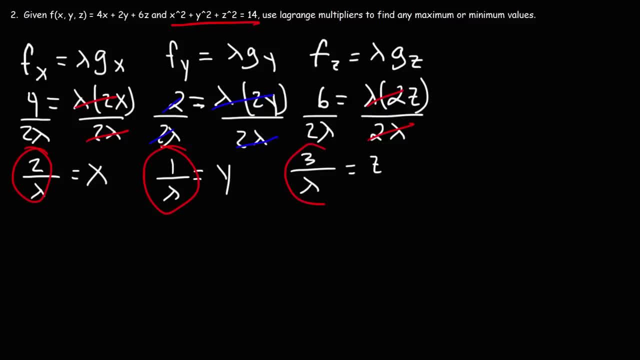 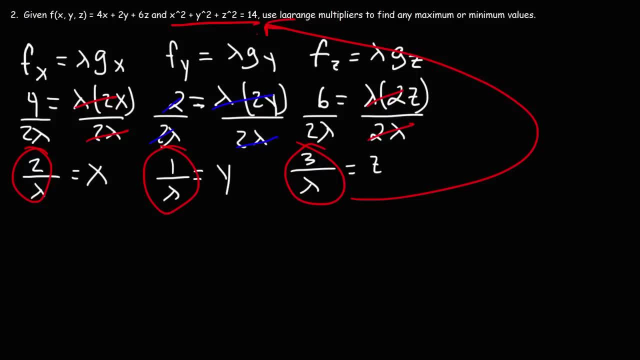 So now we have x, y and z in terms of lambda lambda, So let's go ahead and do that. So instead of x squared, it's going to be 2 over lambda squared, And then, instead of y squared, it's going to be 1 over lambda squared, And then plus z. 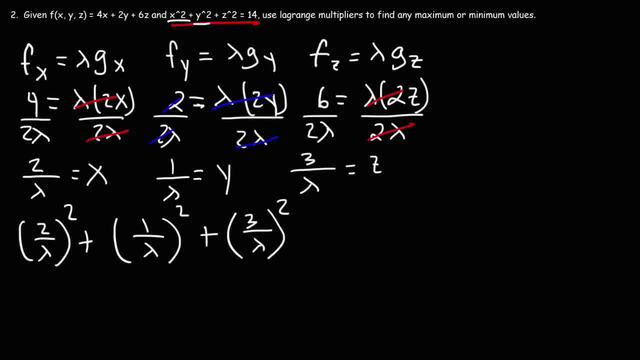 squared, which is 3 over lambda squared, And that's equal to k, which is 14.. So 2 squared is 4.. So this is going to be 4 over lambda squared, And then plus 1 over lambda squared, 3 squared is: 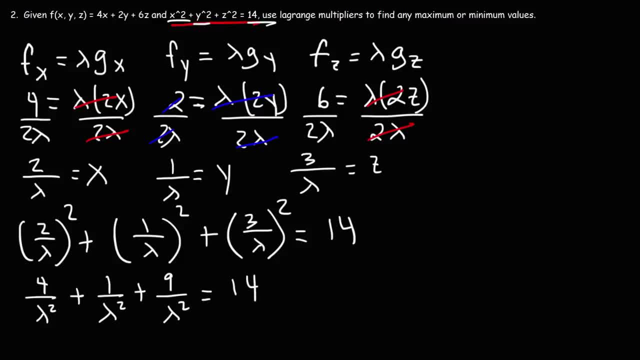 9. And that's equal to 14.. So adding the numerators, we have 1 plus 9, which is 10, plus 4, that's 14. So 14 over lambda squared is equal to 14.. 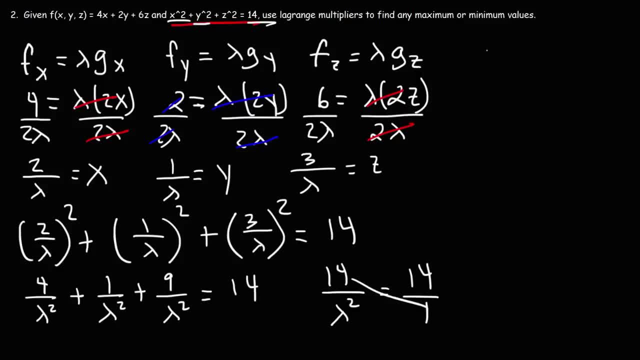 And we can put this over 1 and cross multiply. So 14 times 1 is 14.. And then that's equal to 14 lambda squared. So dividing both sides by 14, we see that lambda squared is equal to 1.. And then, if we take the 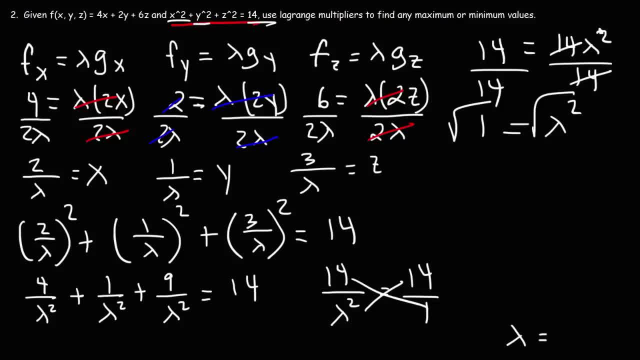 square root of both sides, lambda is going to be plus or minus 1.. So we have two answers for lambda in this example. So let's talk about what we're going to do with that. But first let's free up some space. 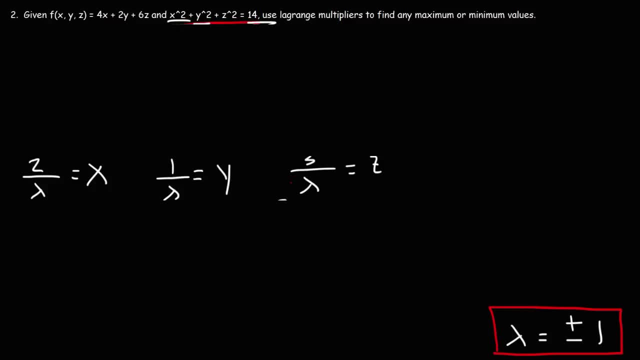 Now, if lambda is equal to 1, x is going to be 2 over lambda, or 2 divided by 1, which is 2.. Y is 1 over lambda, 1 divided by 1, that's 1.. And z is 3 over lambda, which will 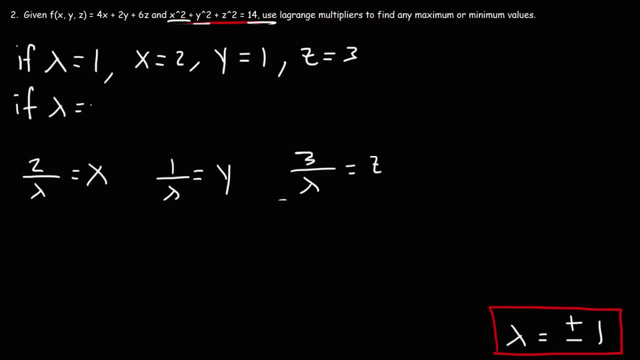 be 3.. Now, if lambda is negative, we're going to have 2 over lambda, or 2 divided by 1, x is going to be negative 2,, y is going to be negative 1, and z is going to be negative 3.. 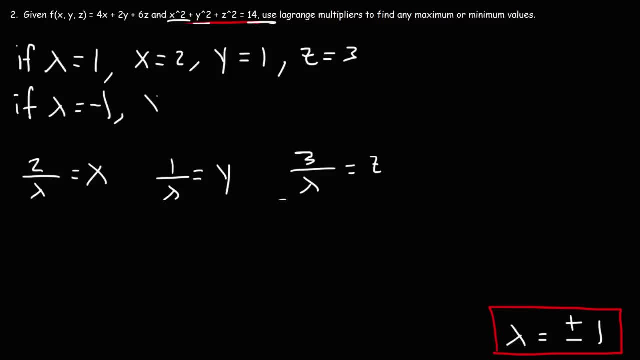 Now, if lambda is negative, 1,, x is going to be negative 2. y is going to be negative 1. And z is going to be negative 3.. Now we need to determine if one of these is the maximum. 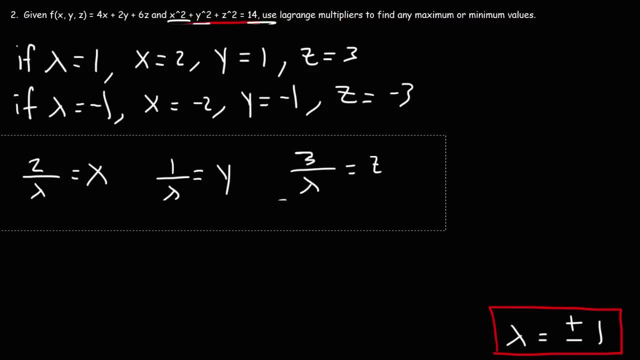 Now we need to determine if one of these is the maximum and, if so, which one, or if both could be a maximum or both could be a minimum. So what we're going to do is plug in each point into the original function. Let's start with the first one. So x is 2, y is 1, z is 3.. 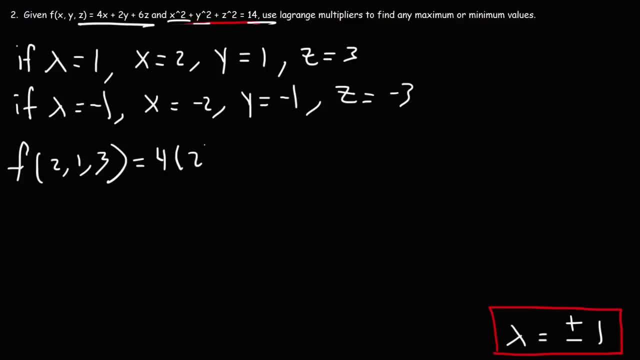 So plugging it into that expression is going to be 4 times 2 plus 2 times 1 plus 6 times 3.. So 4 times 2 is 8, 8 plus 2 is 10, 6 times 3 is 18,, 10 plus 18 is 28.. 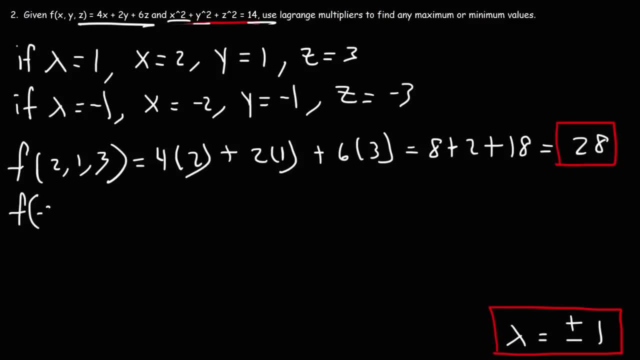 So now let's plug in the other point where x is negative 2,, y is negative 1,, z is negative 3.. So everything is going to be the same, but we're going to get negative 8 plus negative 2 plus. 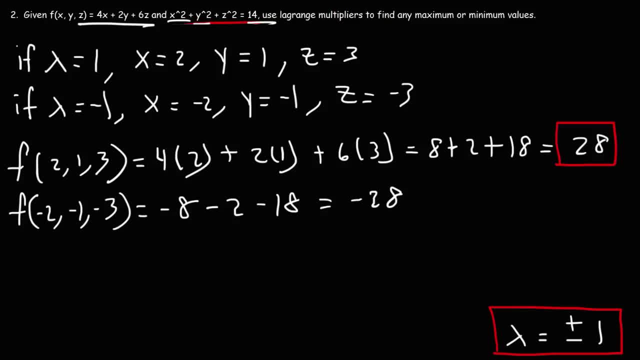 negative 18,, which is going to be negative 28.. That is a terrible looking 2.. Let's do that again So we can clearly see that negative 28 is a minimum and positive 28 is a maximum. And if you're not sure about that, you can try another point. For instance, let's say: if 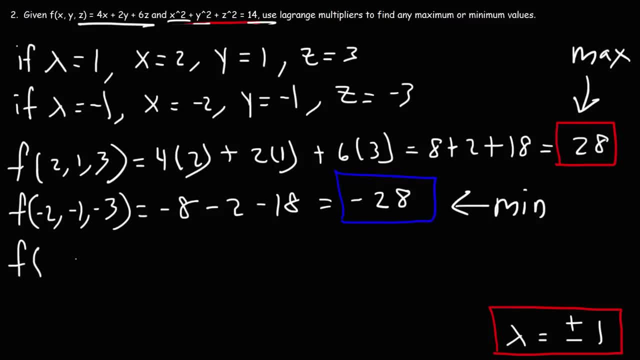 we try the point 3, 1, 2.. Now, before you try this point, you have to make sure that it works with the constraint. So 3 squared plus 1 squared plus 2 squared, that has to equal 14, which it does. 9 plus 1 plus 4 is 14.. 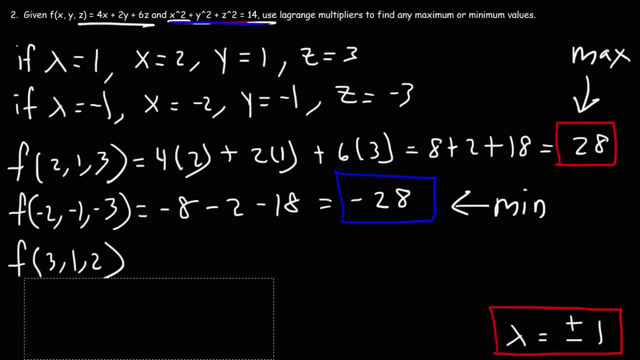 So that equation, or rather that point, lies in the constraint equation. So now plug it in again into our original function f. this is going to be 4 times 3 plus 2 times 1 plus 6 times 2, so that's. 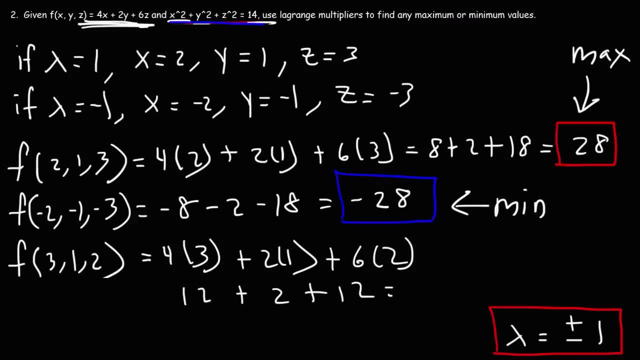 12 plus 2 plus 12.. 12 plus 2 is 14 plus another 12, that's 26.. 26 is less than 28, so that tells us that 28 is indeed a maximum and 26 is much larger than negative 28, which indicates that negative 28. 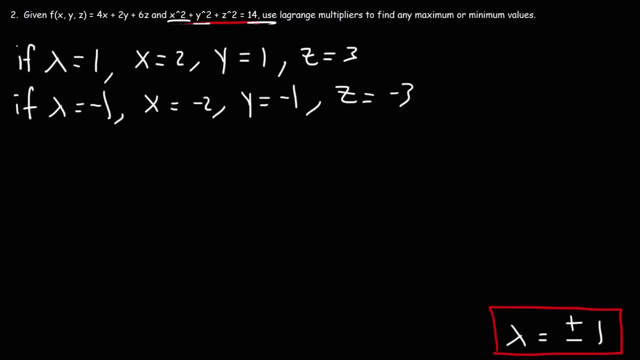 And if so, which one, Or if both. It could be a maximum or both could be a minimum. So what we're going to do is plug in each point into the original function. Let's start with the first one. So x is 2, y is 1, z is 3.. 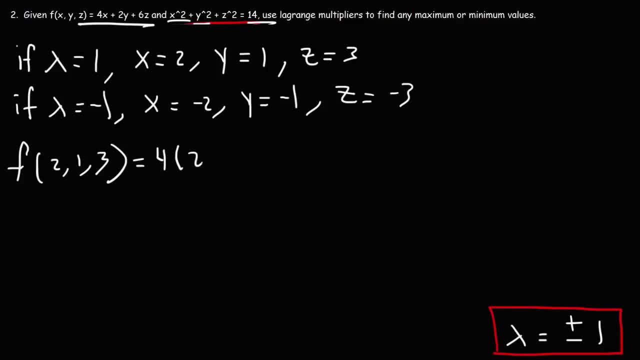 So plugging it into that expression is going to be 4 times 2 plus 2 times 1 plus 6 times 3.. So 4 times 2 is 8.. 8 plus 2 is 10.. 6 times 3 is 18.. 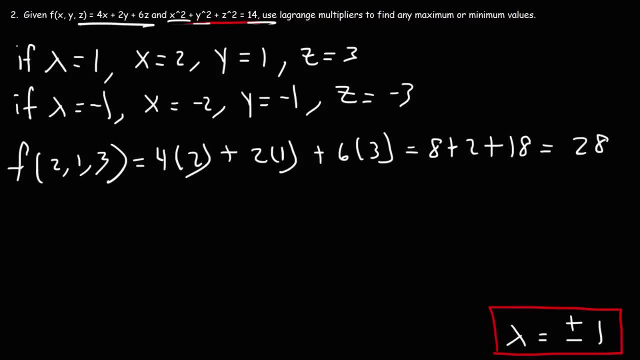 10 plus 18 is 28.. So now let's plug in the other point where x is negative 2,, y is negative 1, z is negative 3.. So everything is going to be the same, but we're going to get negative 8 plus negative 2 plus negative 18,. 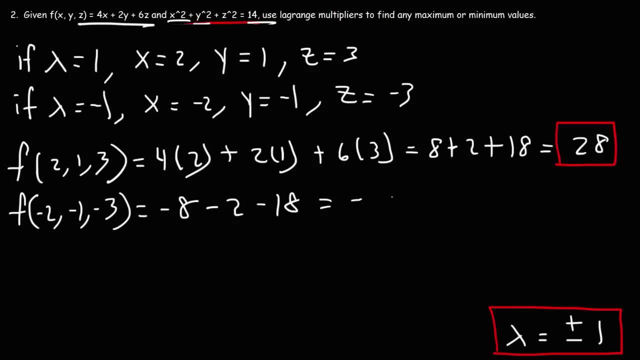 which is going to be negative 28.. That is a terrible looking 2.. Let's do that again So we can clearly see that negative 28, is a minimum and positive 28, is a maximum, And if you're not sure about that, you can try another point. 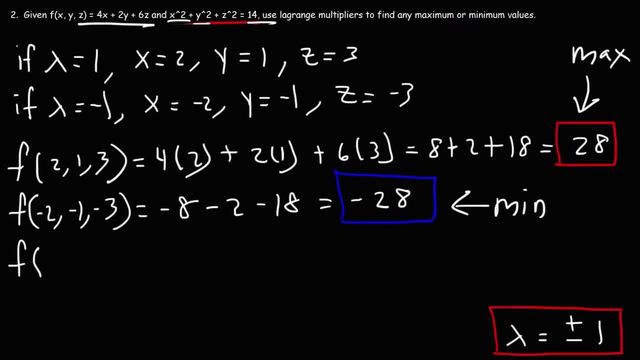 For instance, let's say, if we try the point 3, 1, 2.. Now, before you try this point, you have to make sure that it works with the constraint. So 3 squared plus 1 squared plus 2 squared. 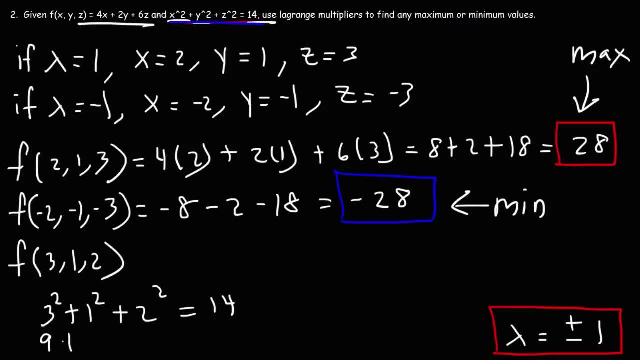 that has to equal 14.. Which it does: 9 plus 1 plus 4 is 14.. So that equation, or rather that point, lies in the constraint equation. So now plug it in into our original function f. This is going to be 4 times 3,. 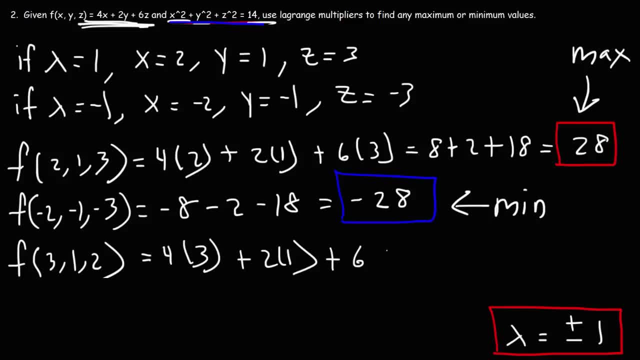 plus 2 times 1, plus 6 times 2.. So that's 12 plus 2 plus 12.. 12 plus 2 is 14, plus another 12.. That's 26.. 26 is less than 28.. 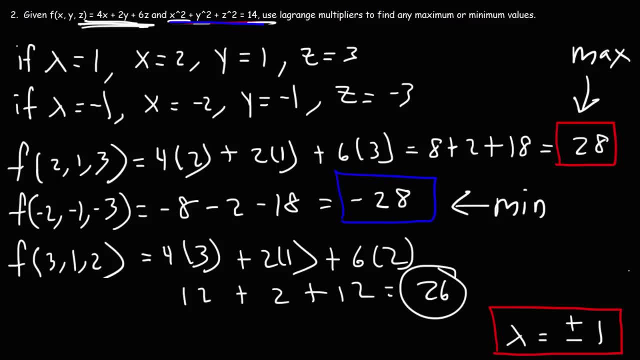 So that tells us that 28 is indeed a maximum And 26 is much larger than negative 28.. Which indicates that negative 28 is a minimum. You can also try another point. You can try f, 1 comma, 2 comma 3.. 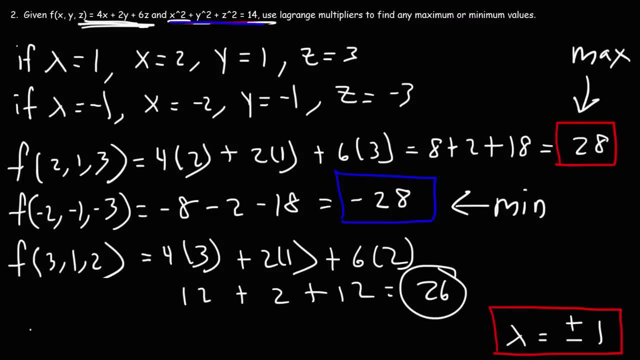 is a minimum. you can also try another point. you can try f 1 comma, 2 comma 3, 1 square plus 2 square plus 3, squared is still 14. so this would be 4 times 1 plus 2 times 2 plus 6 times 3, so that's. 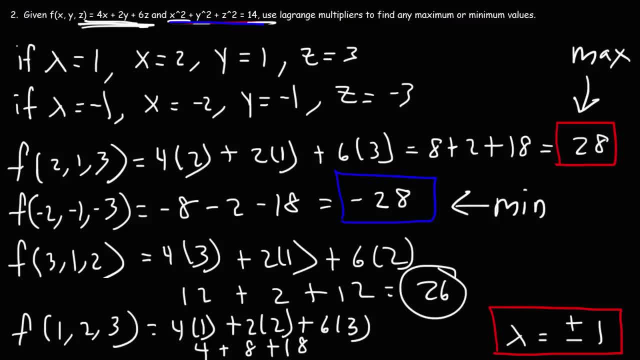 4 plus 8 plus 18.. I took that back 2 times. 2 is 4, not 8.. 4 plus 4 is 8.. 8 plus 18 is 26, which is still less than 28. so 28 is definitely the maximum value of f and negative. 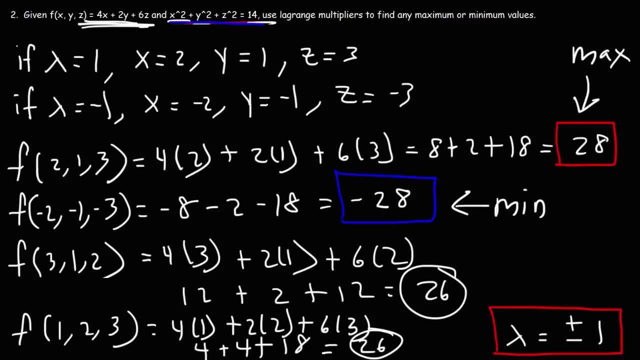 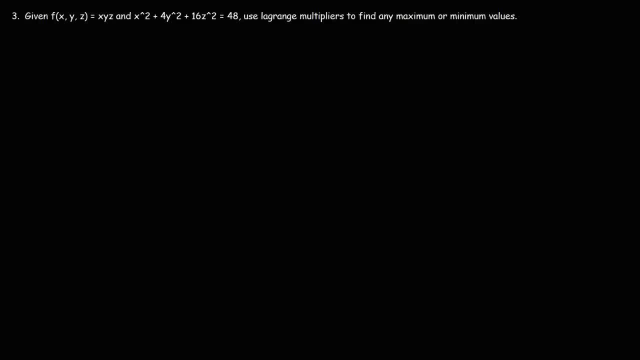 28 is the minimum value of f. so that's it for this problem. now let's move on to number three. this problem is going to be a little bit harder than the previous two, so I recommend that you pause the video and try this problem. once you have the solution, feel free to play it and see. 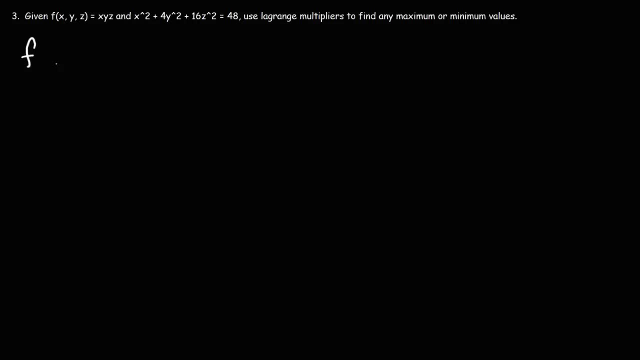 if you have the right answer, so let's begin. we're going to follow the same process that we use in the first two examples, so let's set fx equal to lambda times gx. so what is the derivative of x, y, z with respect to x? the derivative of x is 1, and then we're going to leave the constant alone, yz. 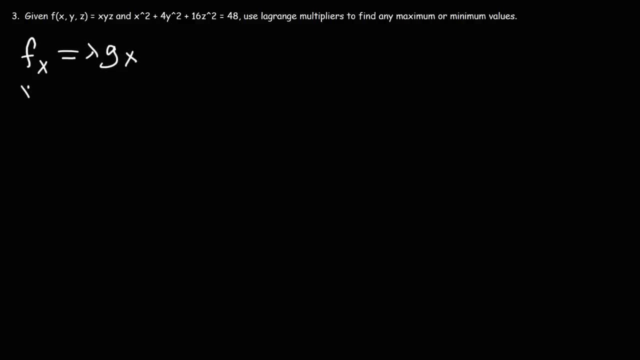 so we're just going to get yz for the partial derivative of f with respect to x. that's going to equal lambda times gx. the derivative of x squared is 2x. now what do you recommend that we do at this point? because we can't really solve for x, because there's 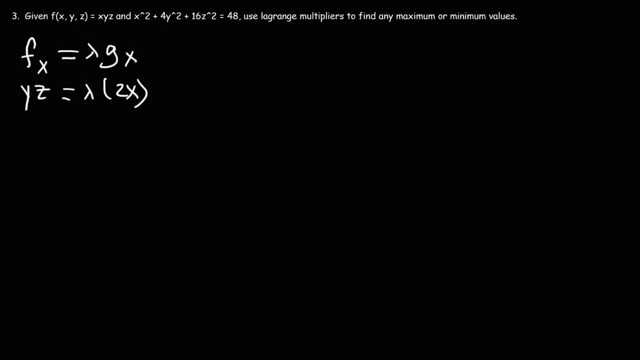 four variables in this equation. we have x, y and z. so in this situation I recommend isolating lambda. so let's divide both sides by 2x. we're going to get lambda by itself. so yz divided by 2x is equal to lambda. now let's move on to our next equation. fy is equal to lambda times gy. 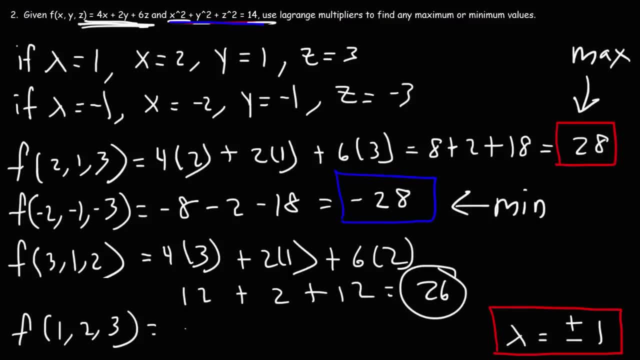 1 squared plus 2 squared plus 3 squared is still 14.. So this would be 4 times 1 plus 2 times 2 plus 6 times 3.. So that's 4 plus 8 plus 18.. I took that back. 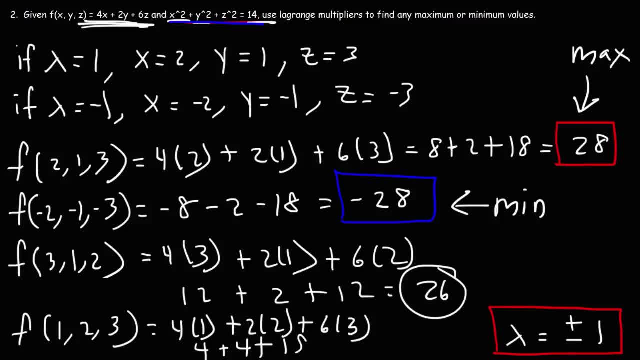 2 times 2 is 4,, not 8.. 4 plus 4 is 8.. 8 plus 18 is 26. Which is still less than 28.. So 28 is definitely the maximum value of f And negative 28 is the minimum value of f. 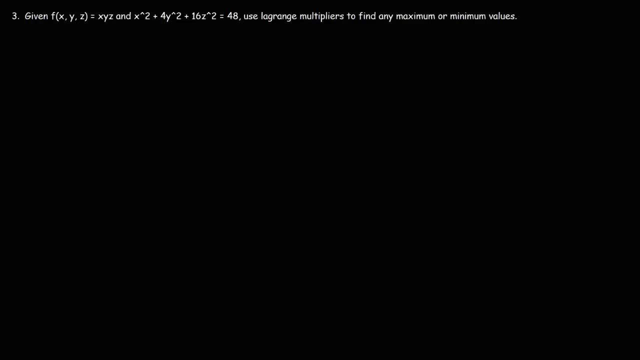 So that's it for this problem. Now let's move on to number 3.. This problem is going to be a little bit harder than the previous two, So I recommend that you pause the video and try this problem Once you have the solution. 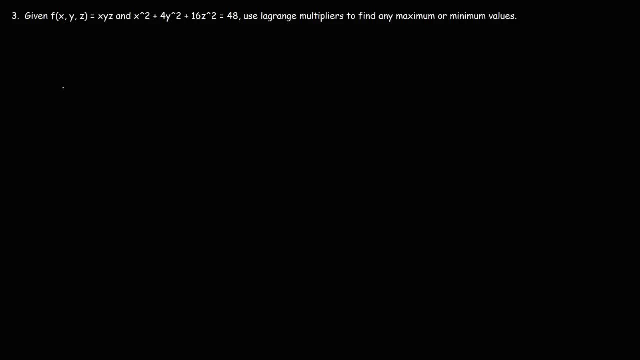 feel free to play it and see if you have the right answer. So let's begin. We're going to follow the same process that we used in the first two examples. So let's set f equal to lambda times g. So what is the derivative of x, y, z with respect to x? 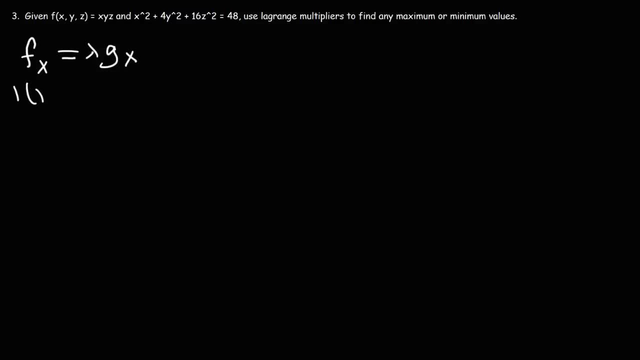 The derivative of x is 1.. And then we're going to leave the constant alone, y z. So we're just going to get y z for the partial derivative of f with respect to x. That's going to equal lambda times g. 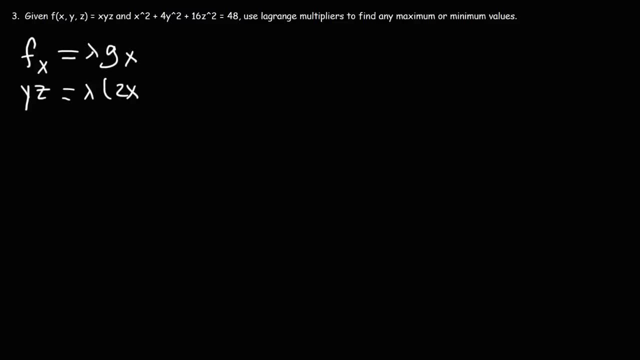 The derivative of x squared is 2x. Now what do you recommend that we do at this point? Because we can't really solve for x, because there's four variables in this equation. We have x, y and z. So in this situation, 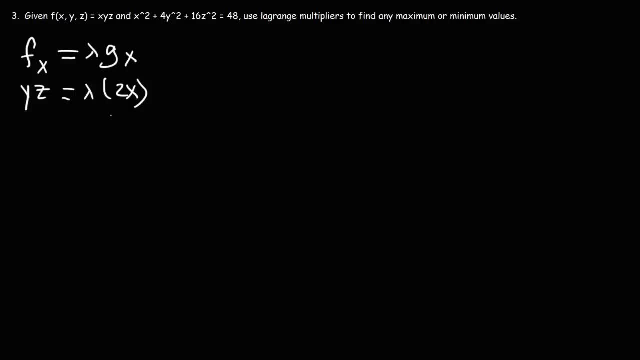 I recommend isolating lambda. So let's divide both sides by 2x. We're going to get lambda by itself. So y z divided by 2x is equal to lambda. Now let's move on to our next equation: f- y is equal to lambda times g. 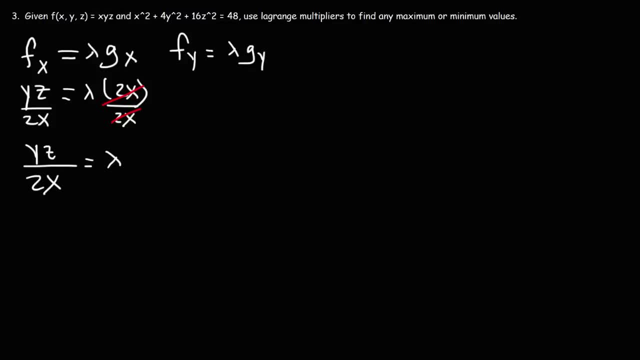 so the derivative of y is 1 times xz. so fy is going to equal xz and gy. the derivative of 4y is going to be 4 times 2y or 8y. so, solving for lambda, we are going to divide both sides by 8y. 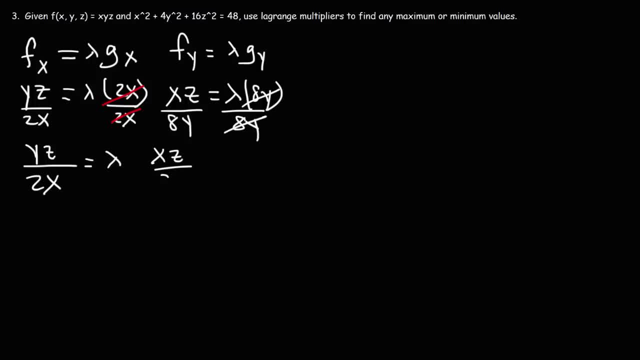 so xz divided by 8y is equal to lambda. now let's move on to the next one. fz is equal to lambda times gz. So the derivative of z is 1 times xymapua2.. So 2y is equal to lambda times gyz. the derivative of 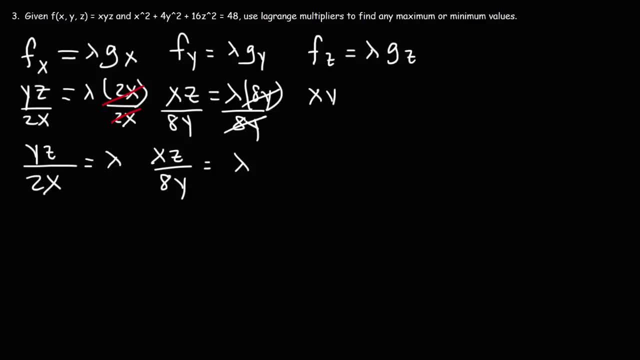 f expression is equal to lambda times gyz. So the derivative of z is 1 times xy, and then this is going to equal lambda. the derivative of 16 times z squared, that's 16 times 2z, which is 32z. Dividing both sides by 32z, we're going to get xy over 32z is equal to. 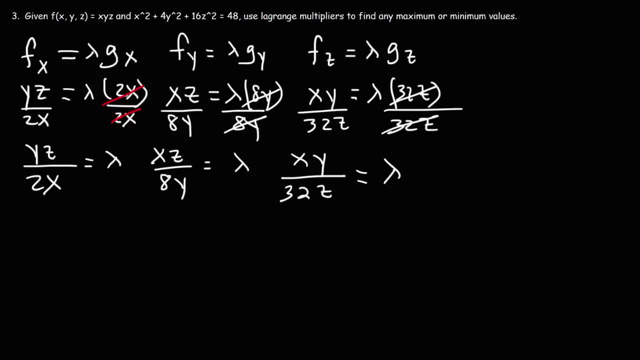 lambda. So now, because each of these three equations equal lambda, they are all equal to each other. So let's call this equation 1,, 2, and 3.. So what I'm going to do is I'm going to set. 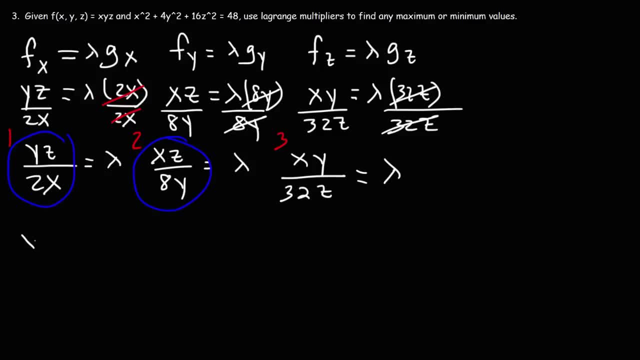 equations 1 and 2 equal to each other. So we have: yz is over 2x is equal to xz over 8y. Notice: by doing this we can cancel out z. If you divide both sides by z, they will cancel. Next we need to cross multiply, So we have y times 8y, which is 8y squared. 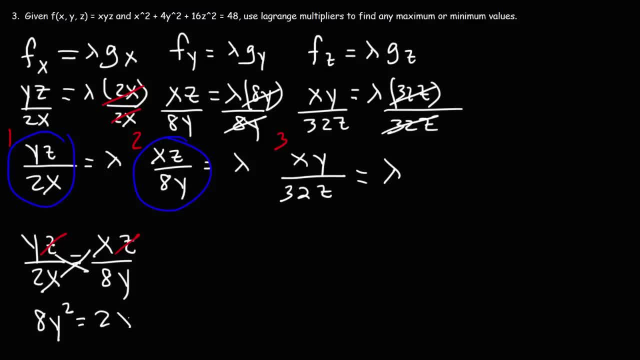 and that's going to be equal to 2x times x, which is 2x squared. Now let's divide both sides by 2.. So this is going to give us 4y squared is equal to xy. I mean, let me say that again. 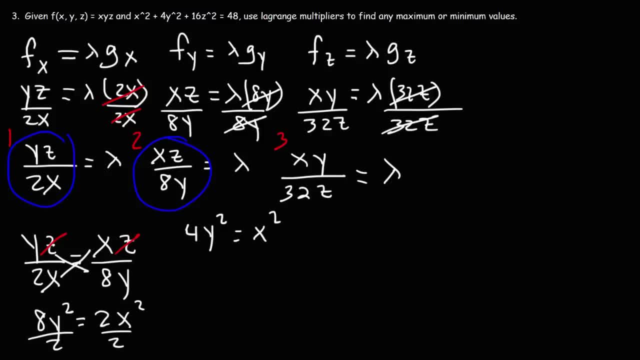 4y squared is equal to x squared, And let's save this equation, because notice that we have it in our constraint. Now let's set equation 2 and equation 3 equal to each other, So this is going to be xz. 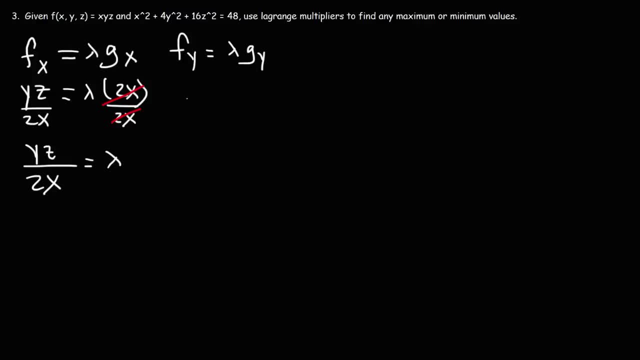 So the derivative of y is 1 times x, z, So f, y is going to equal x, z And g. the derivative of 4y squared is going to be 4 times 2y or 8y, So solving for lambda. 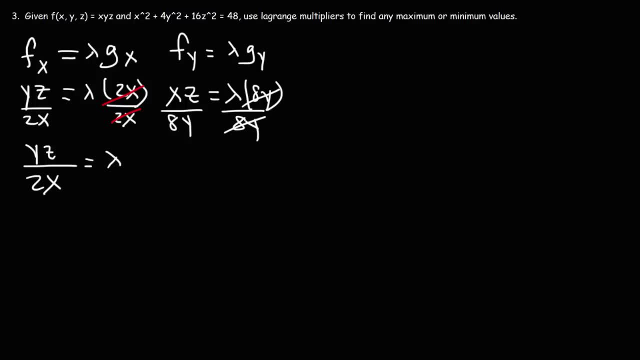 we're going to divide both sides by 8y. So x z divided by 8y And g, the derivative of 4y is equal to lambda. Now let's move on to the next one: f, z is equal to lambda times g- z. 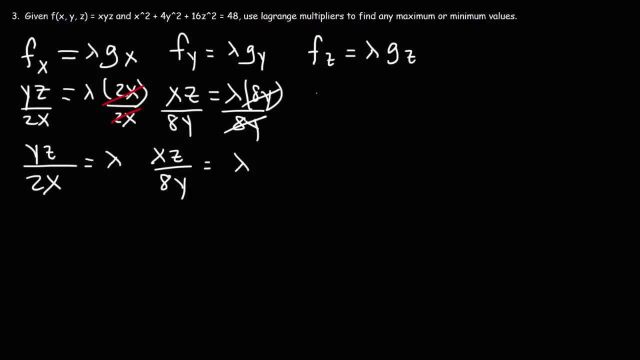 So the derivative of z is 1 times x, y, And then this is going to equal, lambda, The derivative of 16 times z squared, That's 16 times 2z, which is 32z Dividing both sides by 32z. 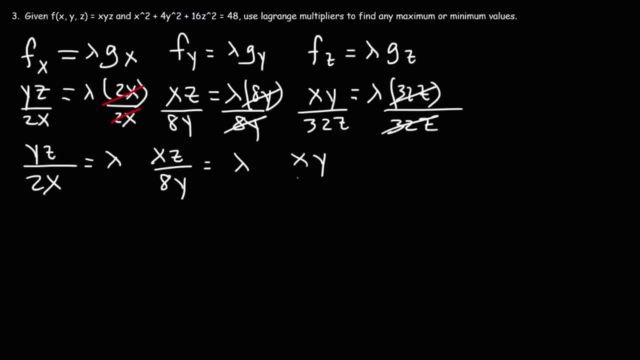 we're going to get x. y over 32z is equal to lambda. So now, because each of these three equations equal lambda, they are all equal to each other. So let's call this equation 1,, 2, and 3.. 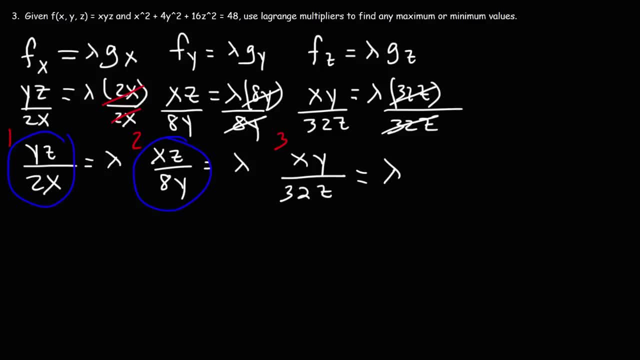 So what I'm going to do is I'm going to set equations 1 and 2 equal to each other, So we have y z over 2x is equal to x z over 8y. Notice, by doing this we can cancel out z. 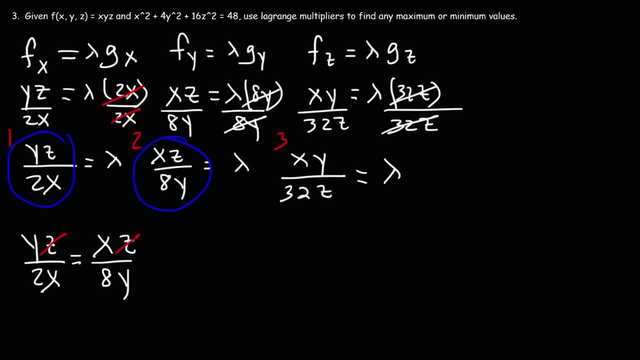 If you divide both sides by z, they will cancel. Next we need to cross multiply, So we have y times 8y, which is 8y squared, And that's going to be equal to 2x times x, which is 2x squared. 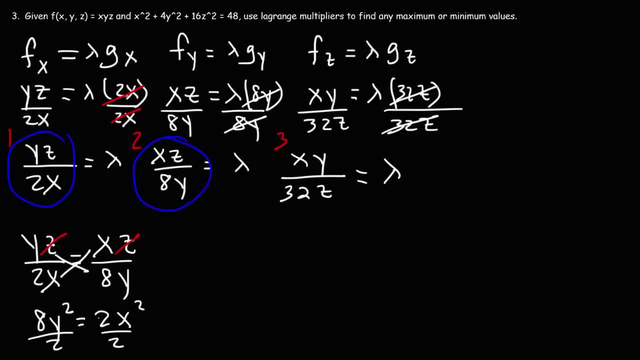 Now let's divide both sides by 2.. So this is going to give us: 4y squared is equal to x squared. I mean, let me say that again: 4y squared is equal to x squared, And let's save this equation. 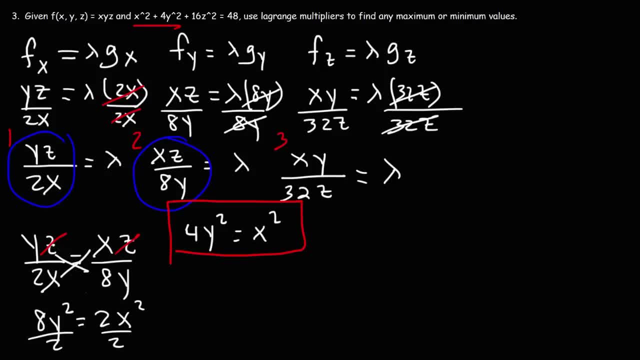 Because notice that we have it in our constraint. Now let's set equation 2 and equation 3 equal to each other, So this is going to be: x. z over 8y is equal to x y divided by 32z. 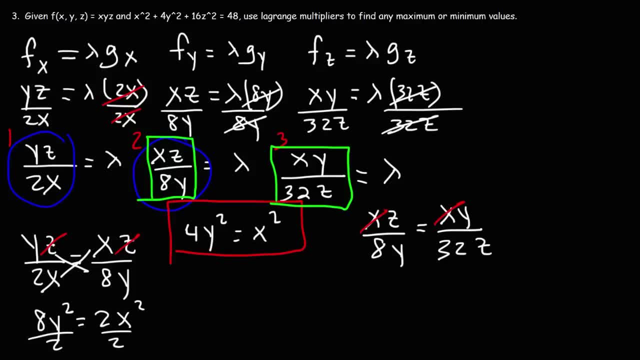 So this time we can cancel out an x And then if we cross multiply, we're going to get 32 times z. squared equals 8y times y or 8y squared. Now I'm going to divide both sides by 2.. 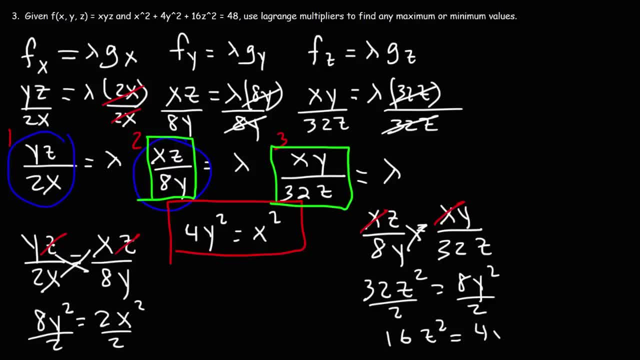 32 divided by 2 is 16.. 8 divided by 2 is 4.. And let's save this expression. Notice that we have both a 16z squared and a 4y squared in the constraint. Now let's replace x squared. 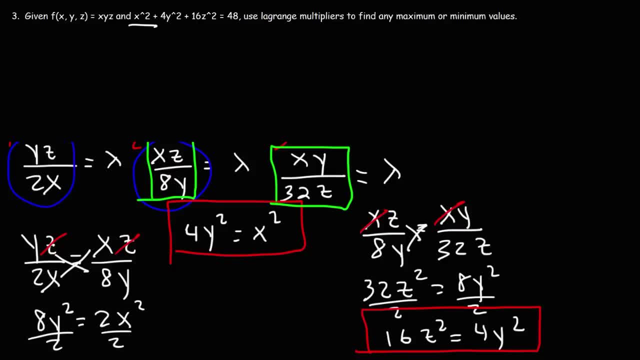 in this equation with 4y squared, because they equal each other. So we're going to have 4y squared and then plus another 4y squared, And then we can replace 16z squared with 4y squared, because they equal each other as well. 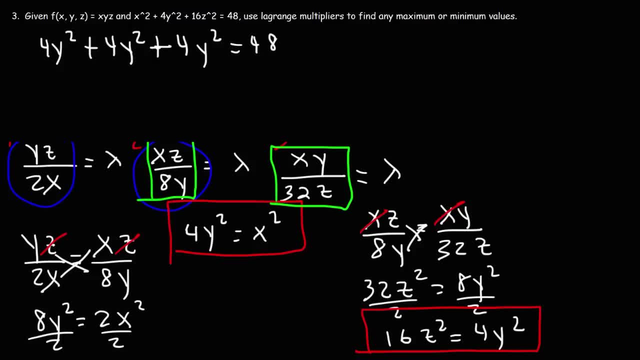 And so this is going to equal 48.. 4 plus 4 plus 4 is the same as 4 times 3,, which is 12.. So we have 12y squared is equal to 48.. Dividing both sides by 12,. 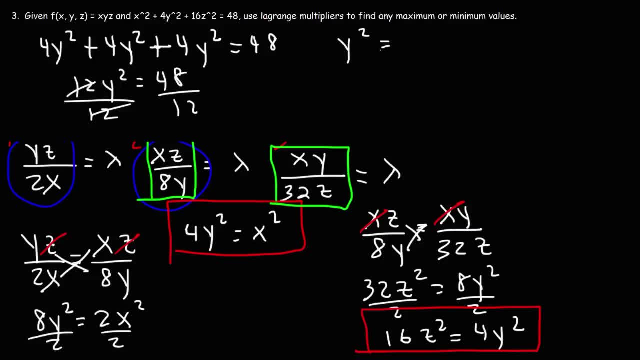 we have: y squared is 48 over 12.. And 48 divided by 12 is 4.. So now we could take the square root of both sides. The square root of 4 is 2, so y can be plus or minus 2.. 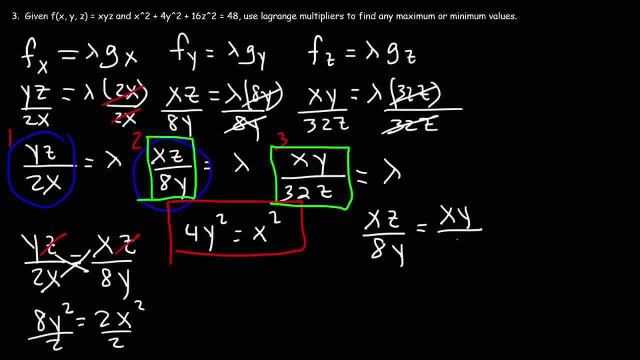 over 8y is equal to xy divided by 32z. So this time we can cancel out an x And then if we cross multiply we're going to get 32 times z squared equals 8y times y or 8y squared. 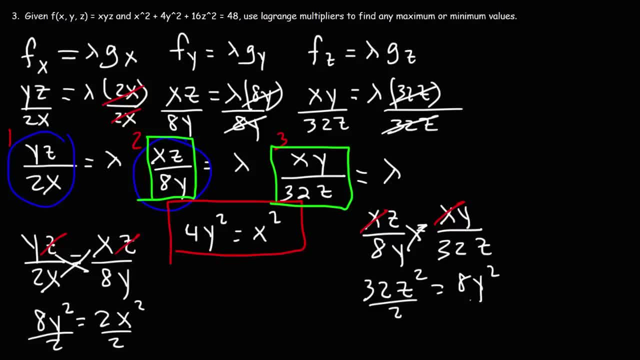 Now I'm going to divide both sides by 2.. 32 divided by 2 is 16,. 8 divided by 2 is 4.. And let's save this expression. Notice that we have both a 16z squared and a 4y squared. 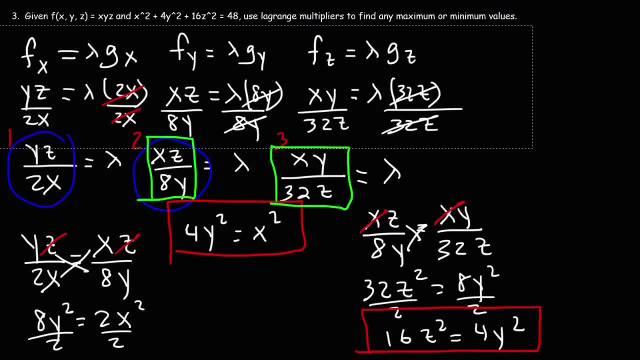 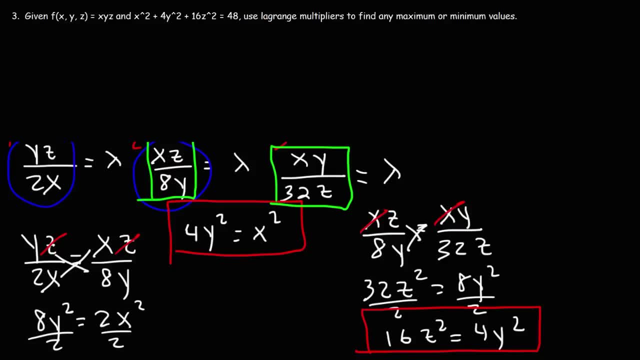 In the constraint. Now let's replace x squared in this equation with 4y squared, because they equal each other. So we're going to have 4y squared and then plus another 4y squared, And then we can replace 16z squared with 4y squared, because they equal each other. 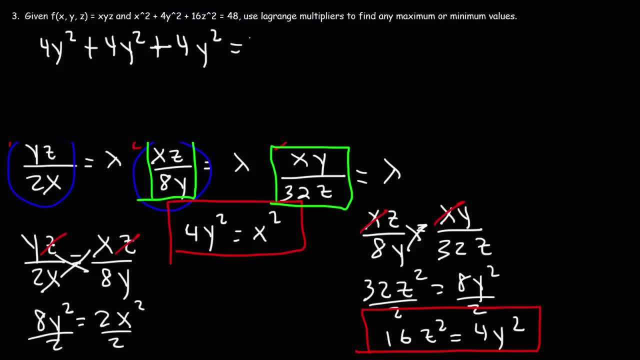 So we're going to have 4y squared and then plus another 4y squared, And so this is going to equal 48.. 4 plus 4 plus 4 is the same as 4 times 3,, which is 12.. 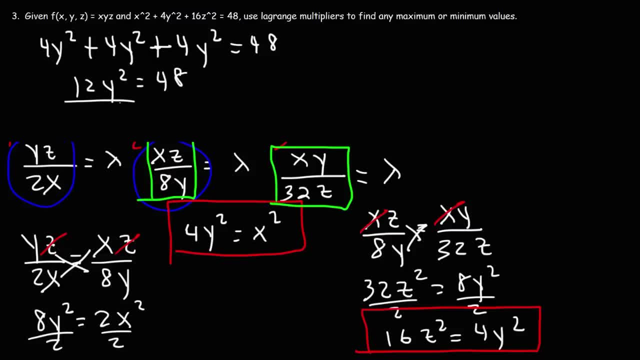 So we have: 12y squared is equal to 48, divided on both sides by 12.. We have y squared is 48 over 12, and 48 divided by 12 is 4.. So now we could take the square root of both sides. 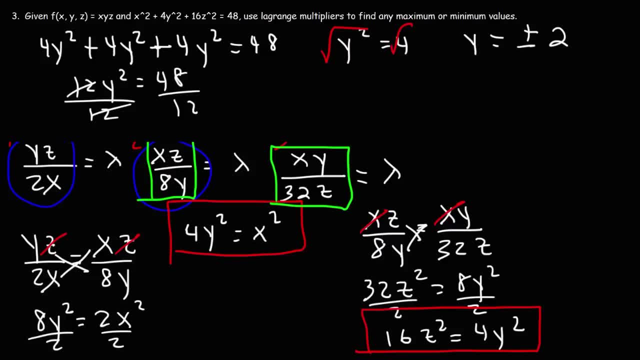 The square root of 4 is 2,, so y can be 4.. Plus or minus 2.. But I'm just going to leave this answer as well. So keep in mind y squared is 4, because we can plug that into this expression. 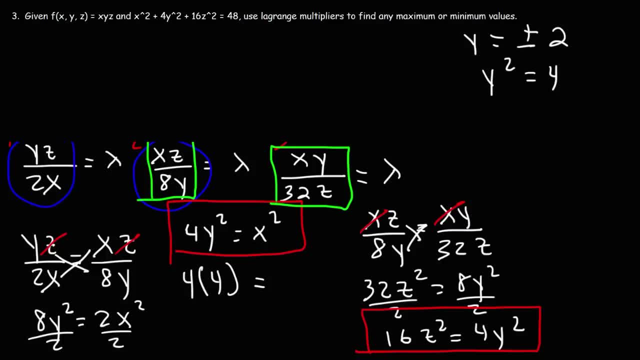 Since y squared is equal to 4, we can replace it with 4.. And so 4 times 4 is 16, and thus we have x squared. Taking the square root of both sides, we get that x is plus or minus 4.. 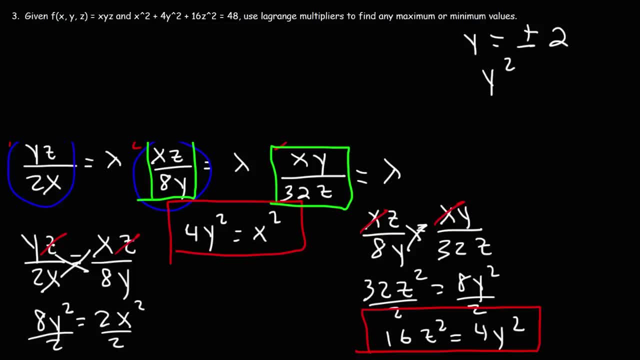 But I'm just going to leave this answer as well. So keep in mind: y squared is 4, because we can plug that into this expression. Since y squared is equal to 4, we can replace it with 4.. And so 4 times 4 is 16,. 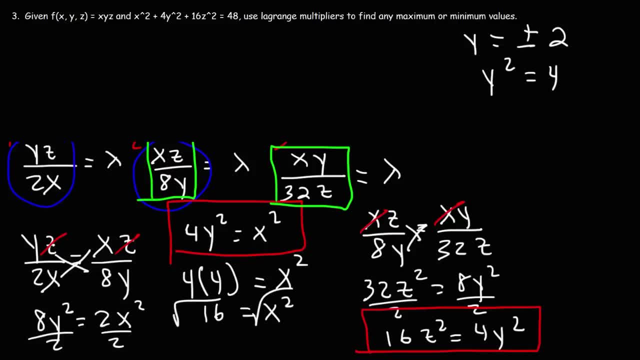 and thus we have x squared. Taking the square root of both sides, we get that x is plus or minus 4.. Now we can plug in y squared into that equation, So we have 16z squared. z squared is equal to 4 times y squared. 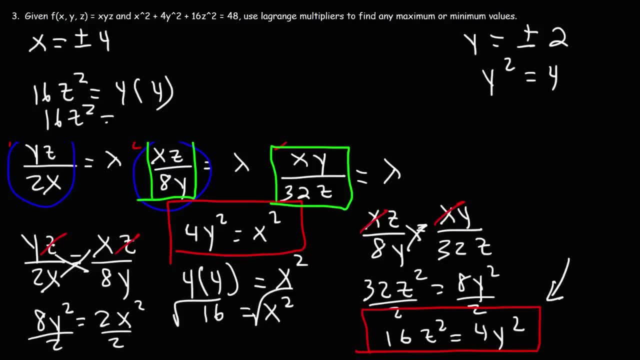 and y squared is 4.. So 16z squared is equal to 16.. Dividing both sides by 16, we get that z squared is 16 over 16, which is 1.. So z is going to be plus or minus 1. 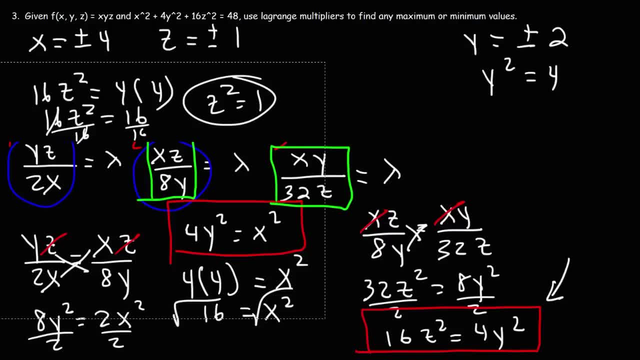 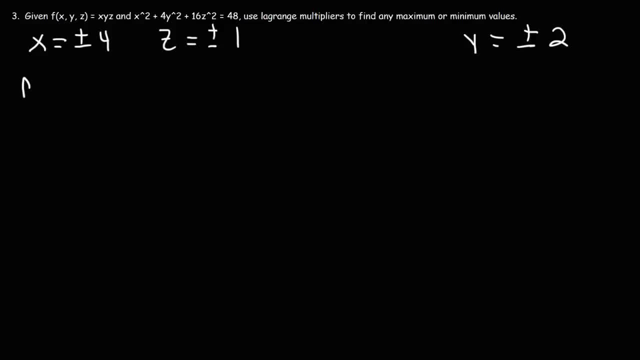 if you take the square root of both sides. So now we have the values of x, y and z. Now let's evaluate the function: when x is positive 4,, when y is positive 2, and when z is positive 1. 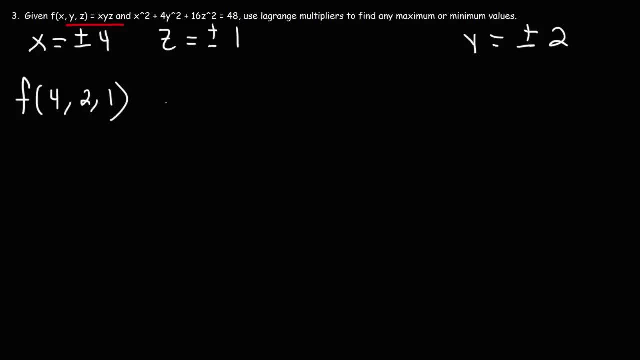 using this expression, x, y, z. So that's going to be 4 times 2 times 1, and that will give us positive 8.. Now we can try evaluating the function at negative 4, negative 2, negative 1.. 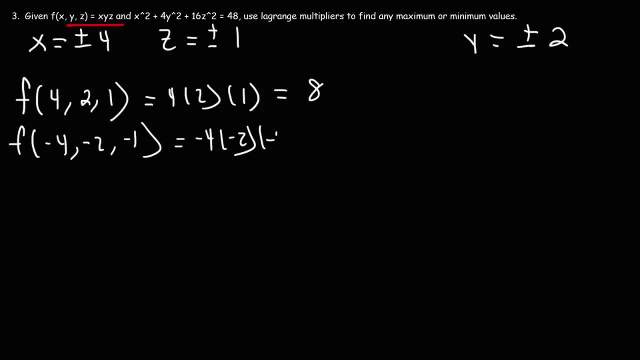 And so that's going to be negative 4 times negative, 2 times negative, 1, which is negative 8.. Now, these are not the only variations that we have for this particular problem. So, for instance, if we were to make a table, 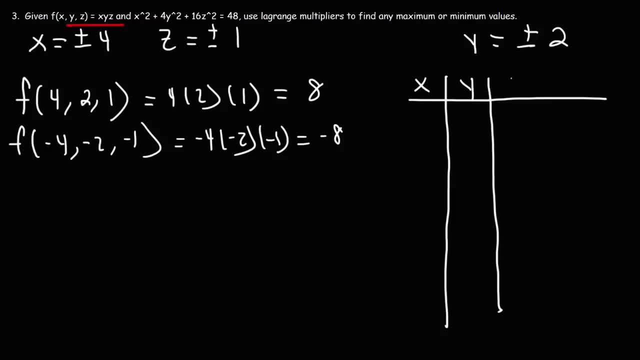 with x, y, z and another column for f. so we see that if x, y and z are all positive, f will be positive 4 times. 2 times 1 is 8. And if they're all negative, 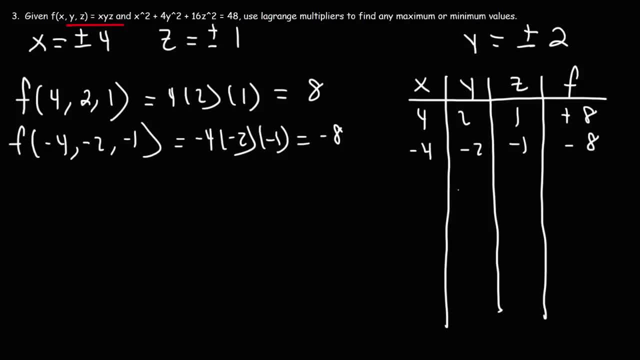 f will be negative. But we can make x positive, y negative and z positive. That will give us negative 8.. And if we plug in these numbers into this expression: x squared plus 4y squared plus 16z squared- 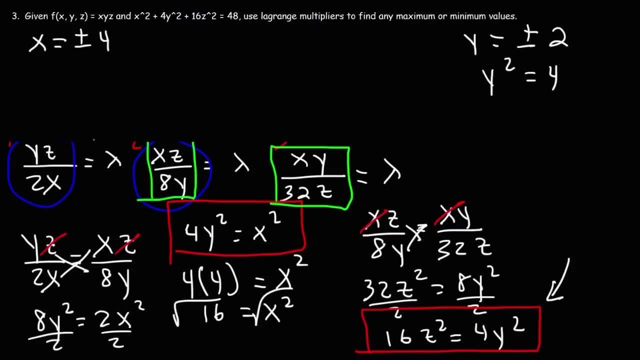 Now we can plug in y squared into that equation. So we have: 16z squared is equal to 4 times y squared, and y squared is 4.. So 16z squared is equal to 16.. Dividing both sides by 16, we get that z squared is 16 over 16, which is 1.. 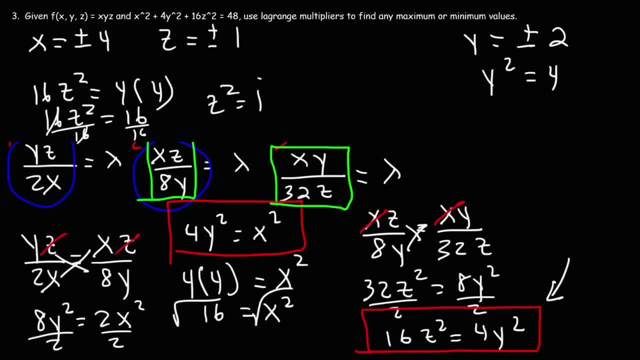 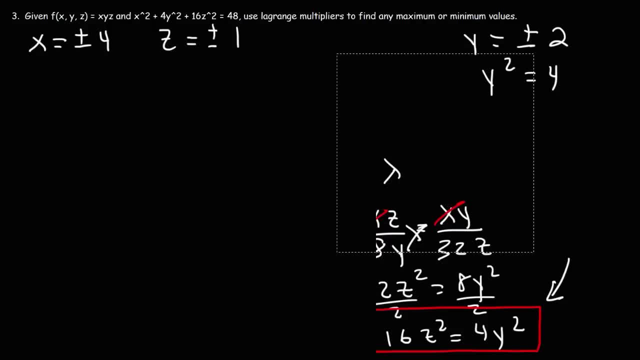 So z is going to be plus or minus 1, if you take the square root of both sides. So now we have the values of x, y and z. Now let's evaluate the function when x is positive: 4,. 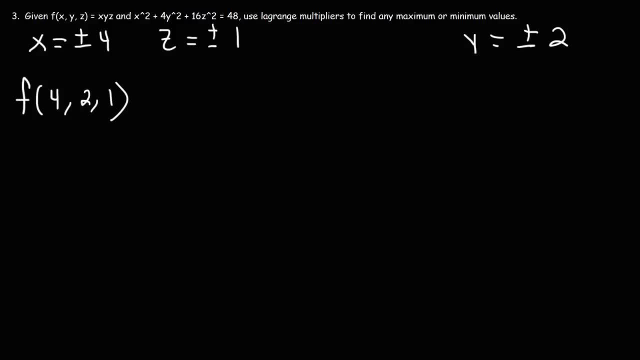 when y is positive 2, and when z is positive 1,. using this expression: x, y, z, So that's going to be 4 times 2 times 1, and that will give us positive 8.. Now we can try evaluating the function at negative 4, negative 2,, negative 1.. 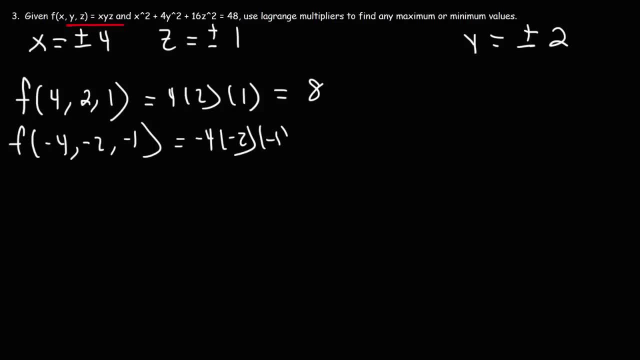 And so that's going to be negative 4 times negative, 2 times negative, 1, which is negative 8.. Now, these are not the only variations that we have for this particular problem. So, for instance, if we were to make a table, 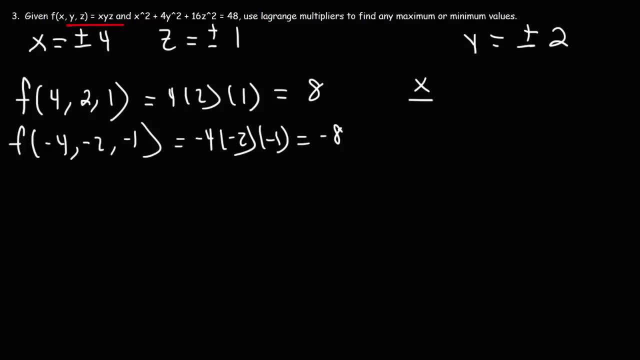 with x, y, z and z, we're going to have x, y, z and another column for f. So we see that if x, y and z are all positive, f will be positive 4 times 2 times 1 is 8.. 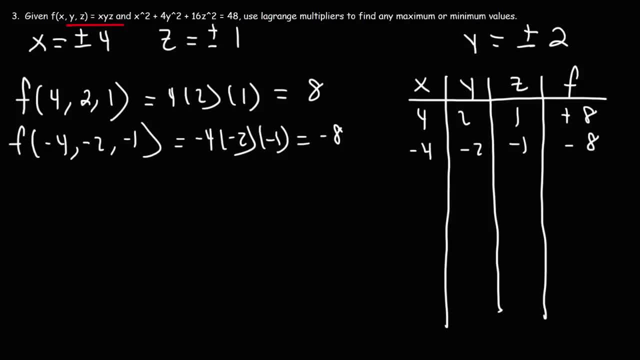 And if they're all negative, f will be negative. But we can make x positive, y negative and z positive. That will give us negative 8.. And if we plug in these numbers into this expression, x squared plus 4y squared, 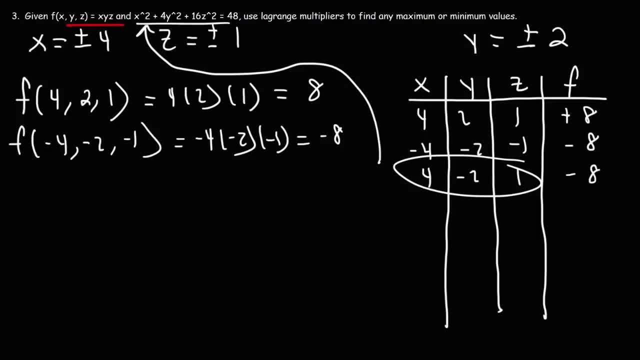 we get negative 8. And if we plug in these numbers into this expression- x squared plus 4y squared plus 16z squared, it's still going to add up to 48.. Because everything is squared, it doesn't matter what the signs are. 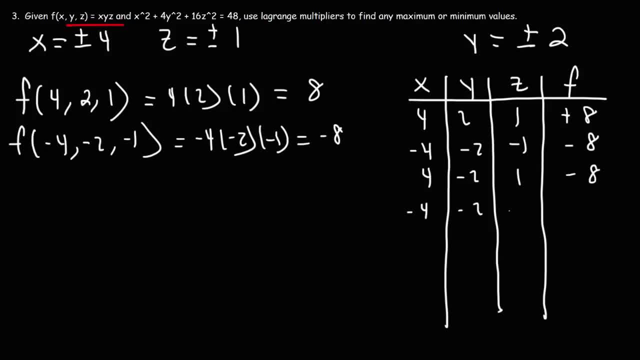 So if I made x negative, y negative and z positive, this will give me positive 8.. Now, because x, y and z can be two things, positive or negative, and we have three variables. we have 2 to the third or 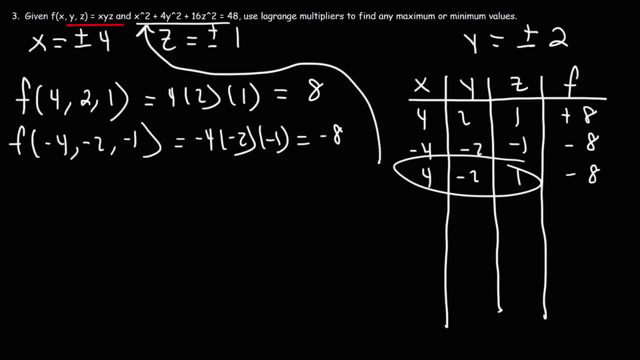 it's still going to add up to 48.. Because everything is squared, it doesn't matter what the signs are. If I made x negative, y negative and z positive, this will give me positive 8.. Now, because x, y and z can be two things. 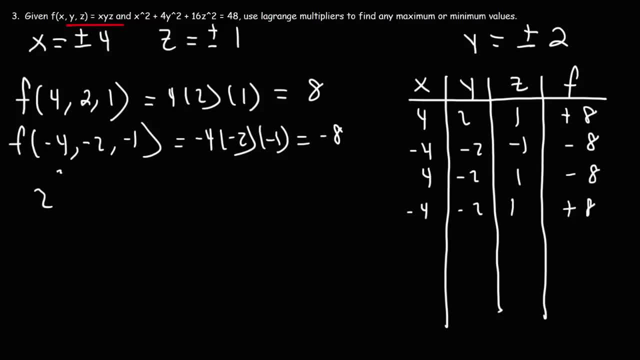 positive or negative and we have three variables. we have 2 to the third or 8, possibilities. Nevertheless, f will be the same, either positive 8 or negative 8.. So when f is equal to positive 8,, 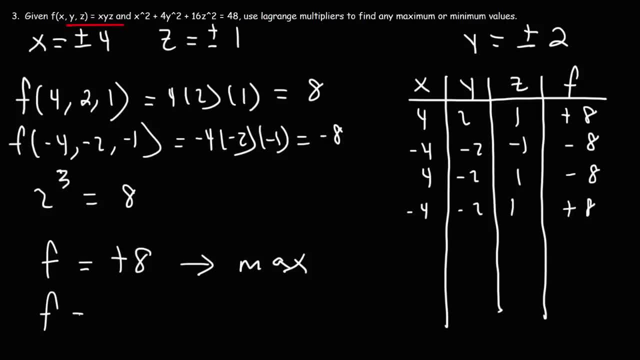 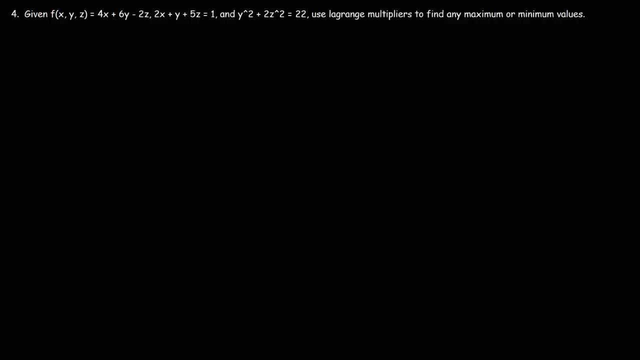 that gives us the maximum value, And when f is equal to negative 8, it's going to give us the minimum value of the function. It's just that there's many points that gives us those minimum and maximum values. So that's all we can do for this problem. 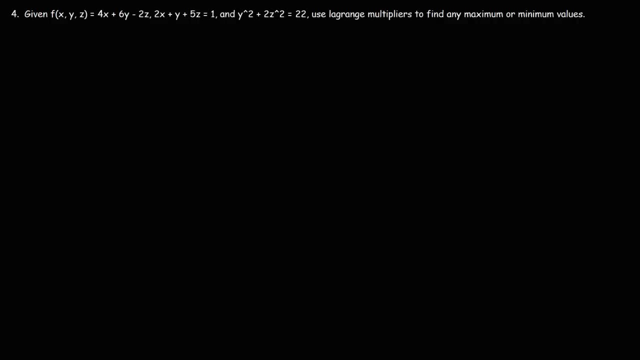 Now let's move on to number 4.. So in this problem we have two constraint equations. This is the first one: 2x plus y plus 5z is equal to 1.. And here we have the second one: y squared plus 2z squared. 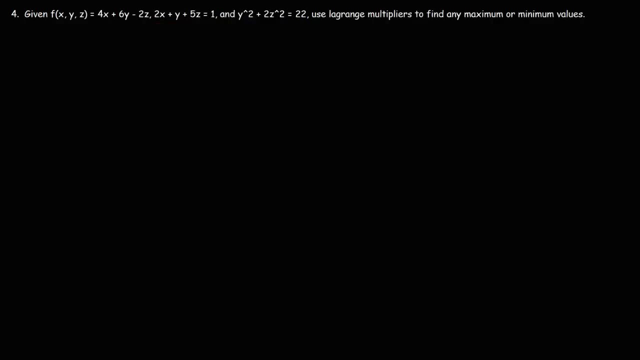 is equal to 22.. So here's some formulas that you need to be aware of. So if we're given some function, f, and we have two constraints, the first one being g, is equal to k and the second one we have h, at some point x, y, z. 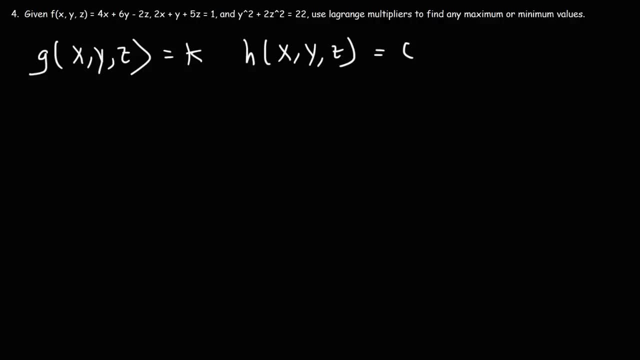 and that's equal to c. Then, in order to write the system of equations, we're going to have: fx is equal to lambda times gx plus u times hx. And then we're going to have: fy is equal to lambda times gy plus uhy. 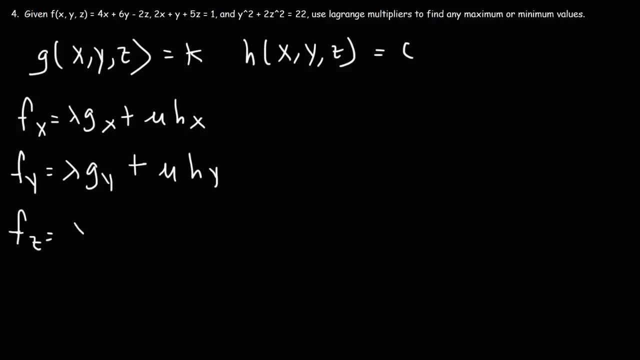 And then fz is equal to lambda gz plus u times hz. So we have five variables that we need to solve: x, y, z, lambda, and a new variable, u. So we need five equations, which we do have it. 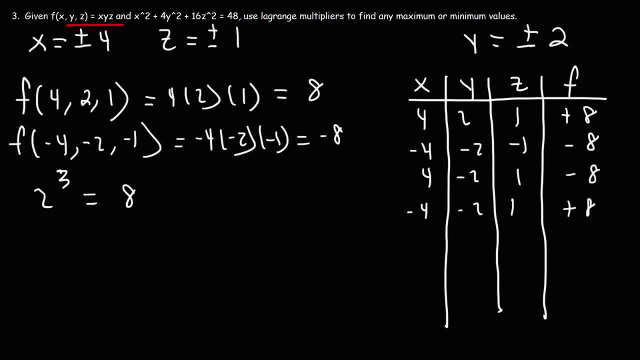 or 8 possibilities. Nevertheless, f will be the same: either positive 8 or negative 8.. So when f is equal to positive 8, that gives us the maximum value, And when f is equal to negative 8, it's going to give us the minimum value of the function. 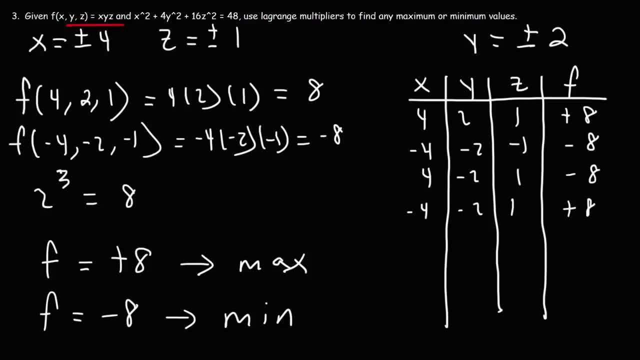 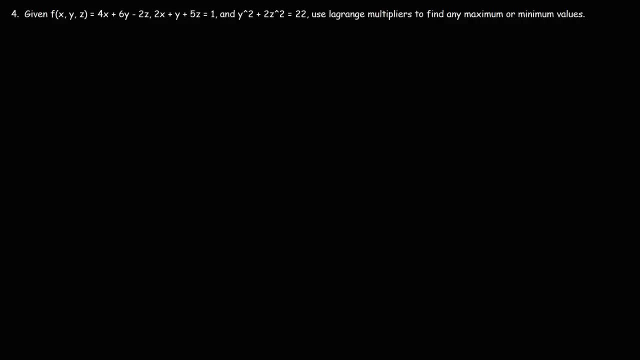 It's just that there's many points. that gives us those minimum and maximum values. So that's all we can do for this problem. Now let's move on to number 4.. So in this problem we have two constraint equations. This is the first one. 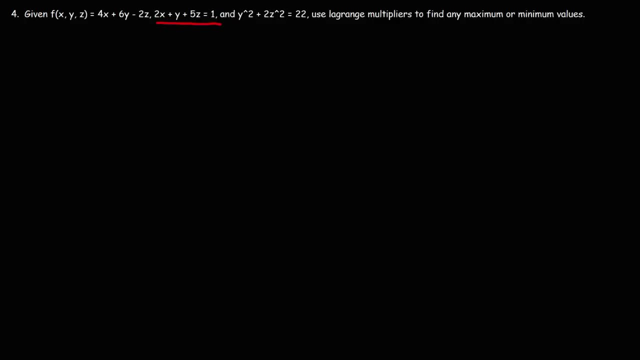 2x plus y plus 5z is equal to 1.. And here we have the second one: y squared plus 2z squared is equal to 22.. So here's some formulas that you need to be aware of. So if we're given some function, f. 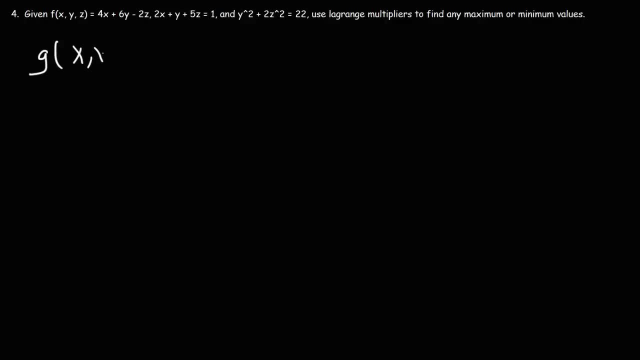 and we have two constraints, the first one being g is equal to k and the second one, we have h, at some point, x, y, z, and that's equal to c. Then, in order to write the system of equations, 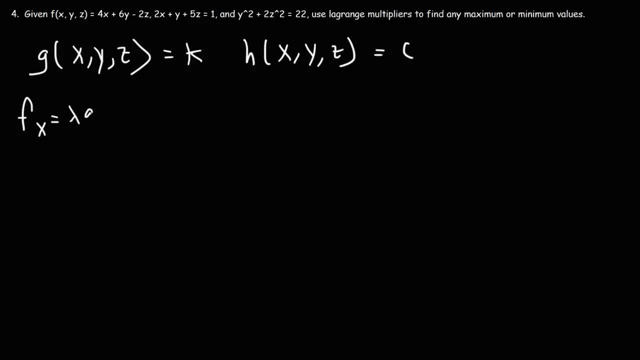 we're going to have: fx is equal to lambda times gx plus u times hx. And then we're going to have: fy is equal to lambda times gy plus u hy, And then fz is equal to lambda gz plus u times hc. So we have five variables. 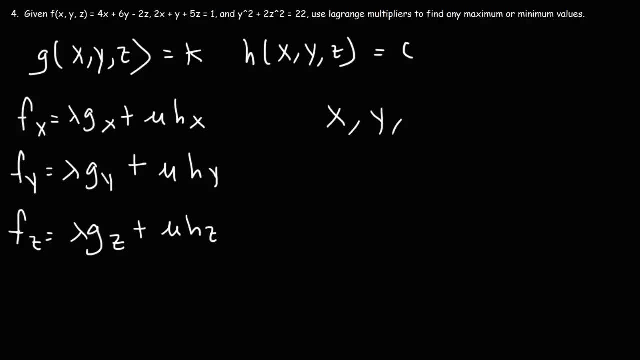 that we need to solve x, y, z, lambda and a new variable, u. So we need five equations, which we do have it: 1,, 2,, 3, 4, 5.. So let's try this problem. 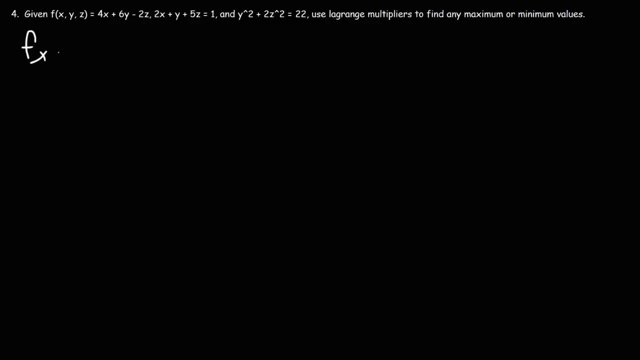 So let's begin with the first partial derivative with respect to x. So we said that's fx is equal to lambda gx plus u times hx. So the derivative of 4x is going to be 4, and that's going to equal lambda. 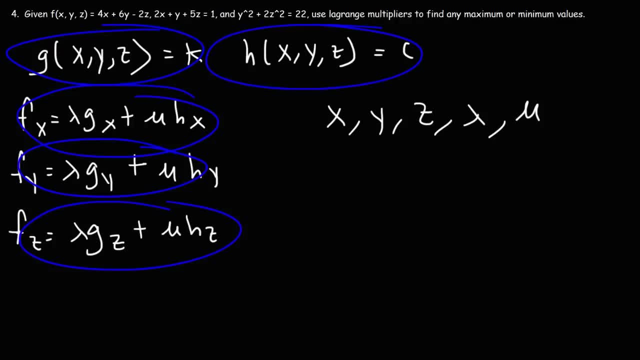 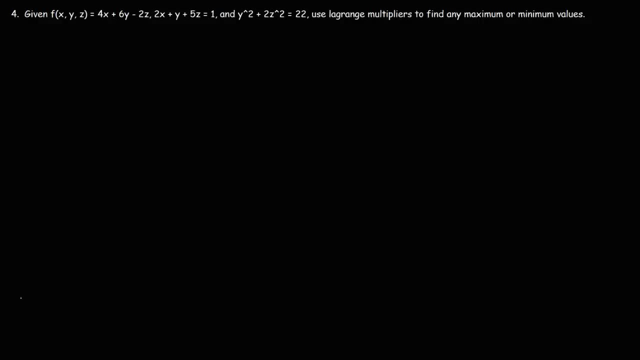 One, two, three, four, five. So let's try this problem. So let's begin with the first partial derivative with respect to x. So we said that's fx is equal to lambda gx plus u times hx, So the derivative of 4x. 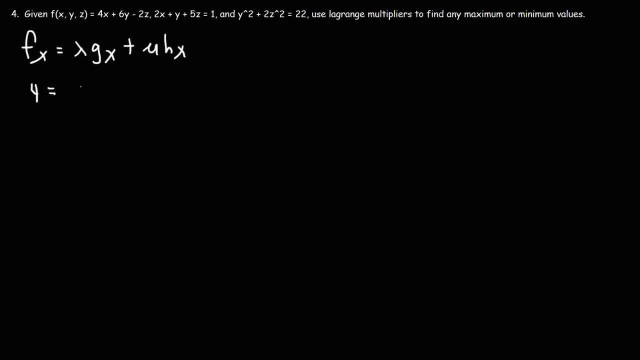 is going to be 4, and that's going to equal lambda. and then this is g- Let me just write that here- And then this is going to be h. So for gx, the derivative of 2x is going to be 2. 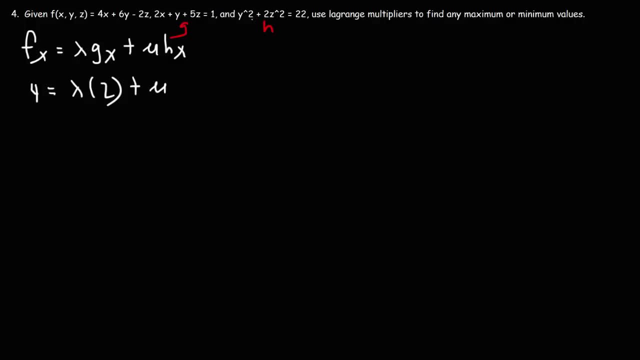 plus u times hx, The derivative of that equation with respect to x is 0, because there are no x variables in that equation. So u times 0 is 0. So we have: 4 is equal to 2 lambda Dividing both sides by 2,. 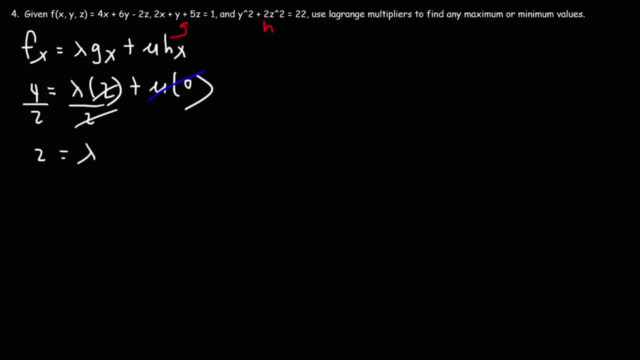 we can see that lambda is equal to 2.. Now let's move on to the next one. So we have gx. is- I mean- I take that back- that's going to be fy, rather, is equal to lambda, gy plus u times hy. 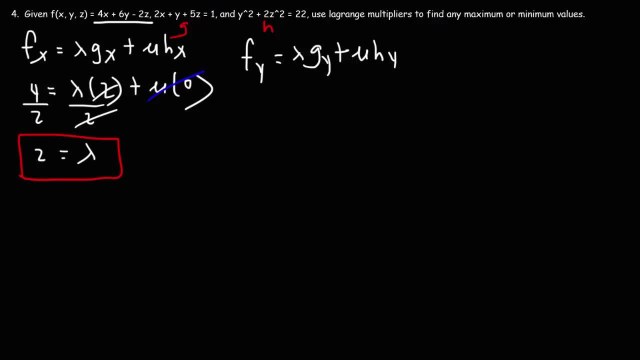 So the derivative of this expression with respect to y, the derivative of 6y, rather, that's going to be 6, and then gy, the derivative of y, is going to be 1.. And then we can replace lambda with 2, since we already know what it is. 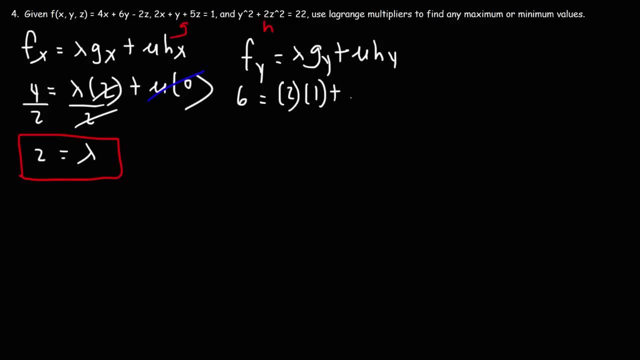 So this is going to be 2 times 1, and then plus u and then hy. So the derivative of y squared is 2y, So we have 6,. if we subtract both sides by 2,, 6 minus 2 is 4,. 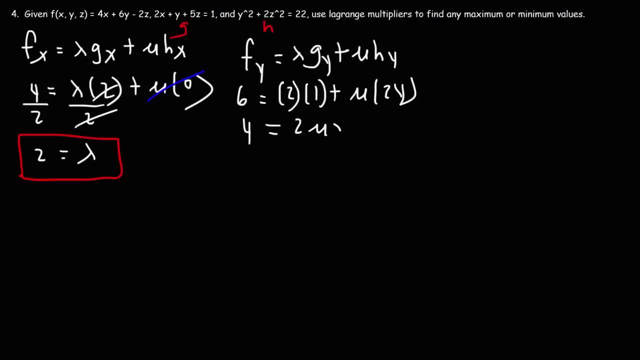 and that's equal to 2 times u times y. What I'm going to do here is I'm going to isolate the y variable, So let's divide both sides by 2 times u, So 4 over 2 is going to be 2.. 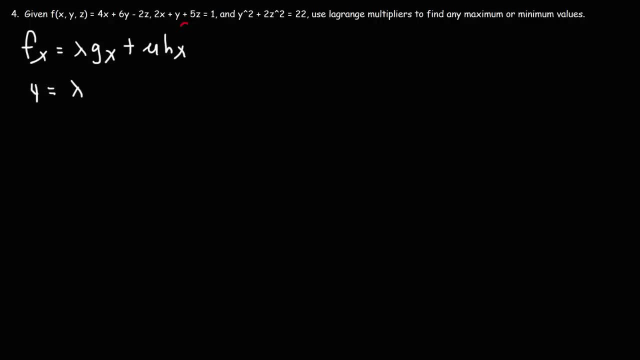 and then this is g- Let me just write that here- And then this is going to be h. So for gx the derivative of 2x is going to be 2 plus u times hx. The derivative of that equation with respect to x is 0,. 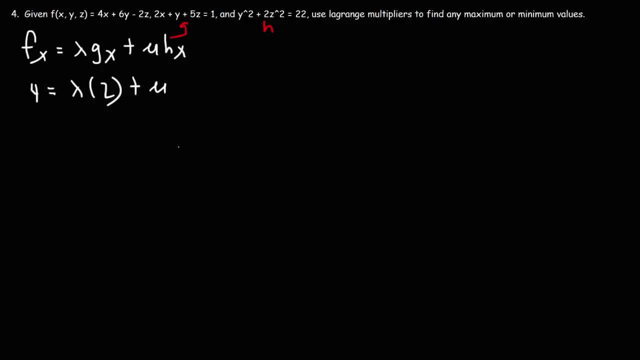 because there are no x variables in that equation. So u times 0 is 0.. So we have: 4 is equal to 2 lambda divided on both sides by 2. We can see that lambda is equal to 2.. Now let's move on to the next one. 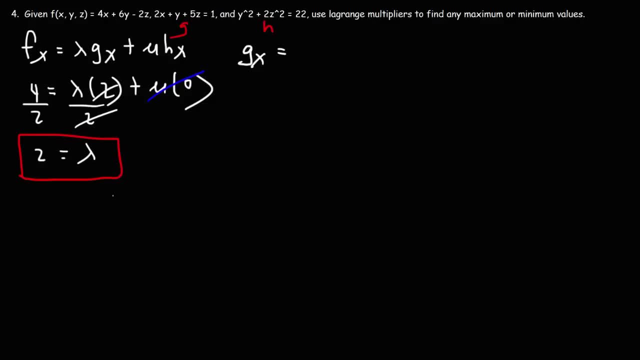 So we have gx is- I mean- I take that back- That's going to be fy, rather- is equal to lambda gy plus u times hy. So the derivative of this expression with respect to y, the derivative of 6y, rather, 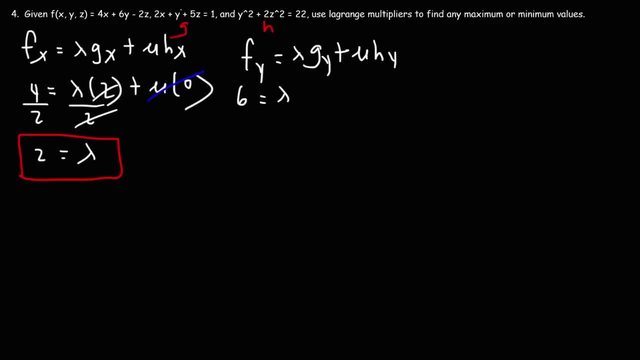 that's going to be 6.. And then gy, the derivative of y, is going to be 1.. And then we can replace lambda with 2, since we already know what it is. So this is going to be 2 times 1,. 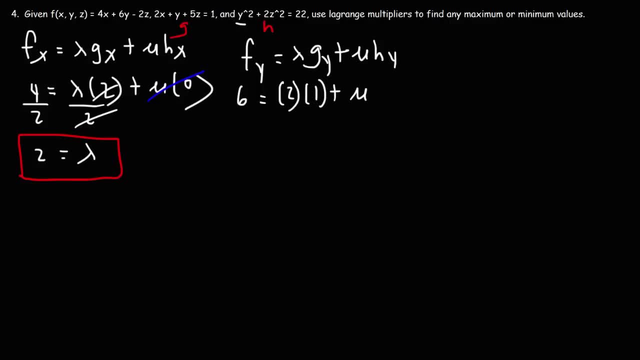 and then plus u and then hy. So the derivative of y squared is 2y, So we have 6.. If we subtract both sides by 2,, 6 minus 2 is 4, that's equal to 2 times u times y. 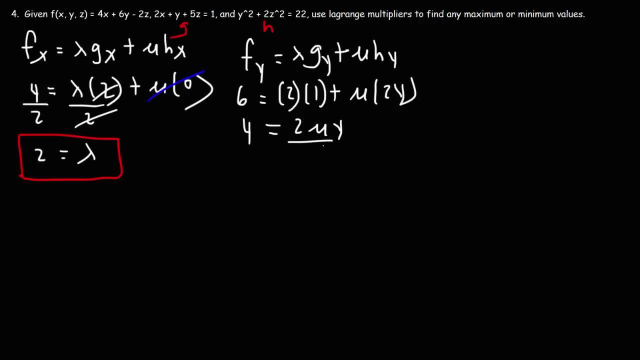 What I'm going to do here is I'm going to isolate the y variable. So let's divide both sides by 2 times u, So 4 over 2 is going to be 2.. So 2 over u is equal to y. 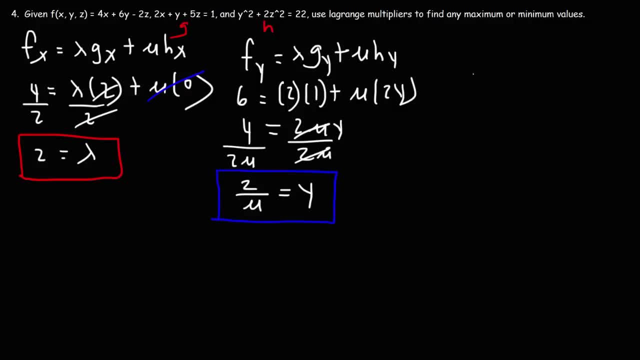 So let's save this equation for later, And now let's move on to our third partial derivative equation with respect to z. So fz, the derivative of negative 2z, is going to be negative 2.. That equals lambda. And then gz. 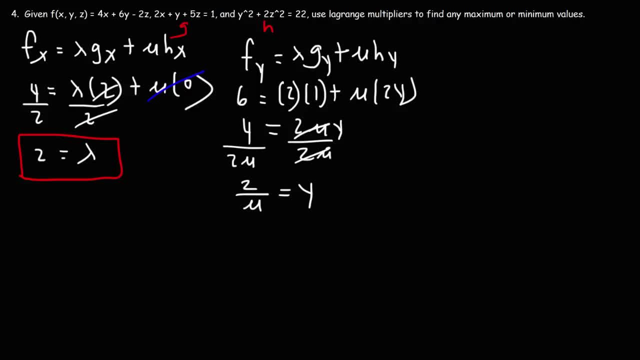 So 2 over u is equal to y. So let's save this equation for later. And now let's move on to our third partial derivative equation with respect to z. So fz, the derivative of negative 2z is going to be negative 2,. 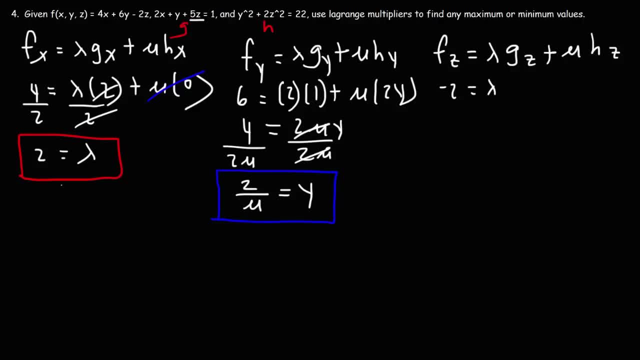 that equals lambda and then gz. the derivative of 5z is: unless you place lambda with 2, so this is going to be 2 times 5, plus u, and then hz. The derivative of 2z squared is going to be 4z. 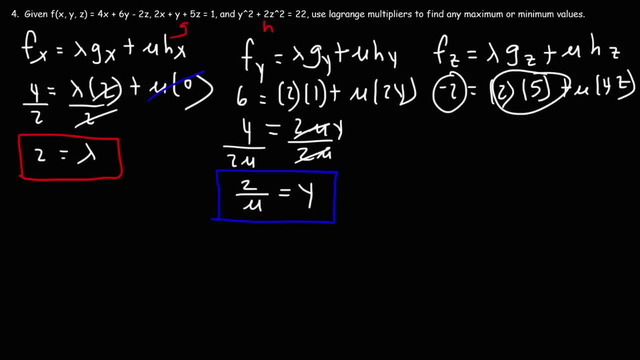 So we have negative 2, 2 times 5 is 10, subtracting both sides by 10, it's going to be negative 2 minus 10, which is negative 12.. So we're going to try to isolate z. 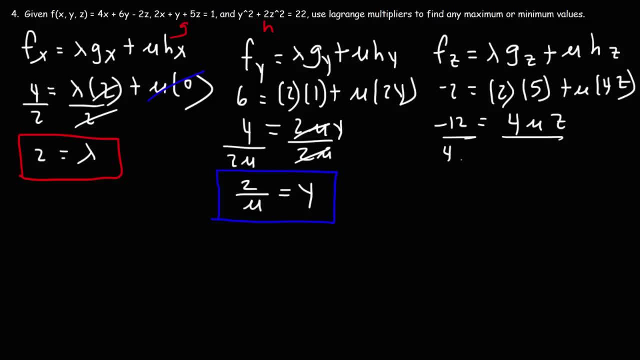 so we're going to divide both sides by 4u: Negative 12 divided by 4 is negative 3.. So we have negative 3 over u is equal to z, And now let's save this expression as well. So notice that we have an equation. 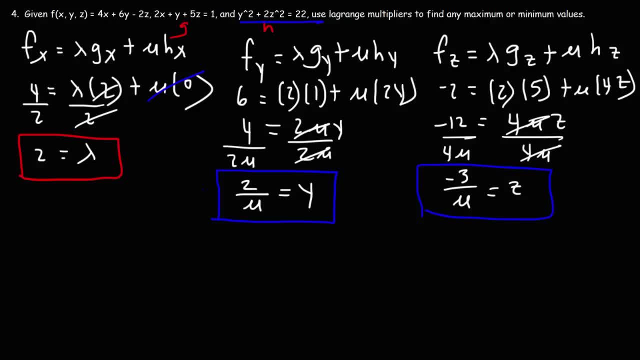 in terms of y and z. So what we're going to do is plug in or replace y with 2 over u and then replace z with negative 3 over u. So we're going to get 2 over u squared and then plus 2z squared. 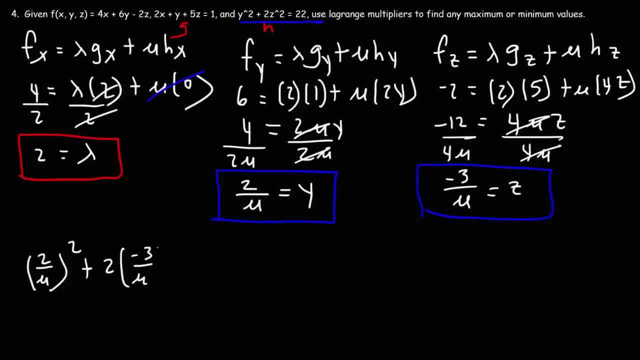 or 2 times negative, 3 over u squared, and that's going to equal 22.. So 2 squared is 4,, 3 squared is 9, 9 times 2 is 18, so that's going to be 18 over u squared. 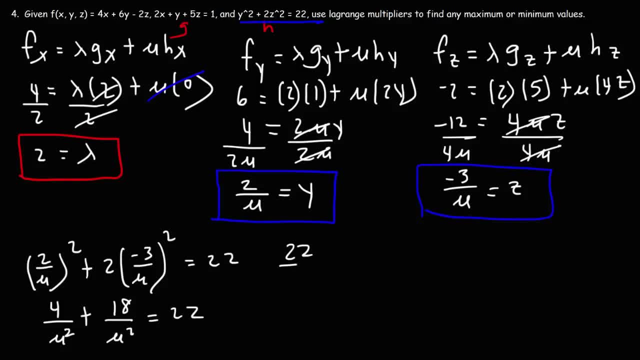 4 plus 18 is 22,. so we have 22 over u squared, which equals 22.. So this means that u squared is 1.. And if u squared is 1, taking the square root of both sides, we can see that 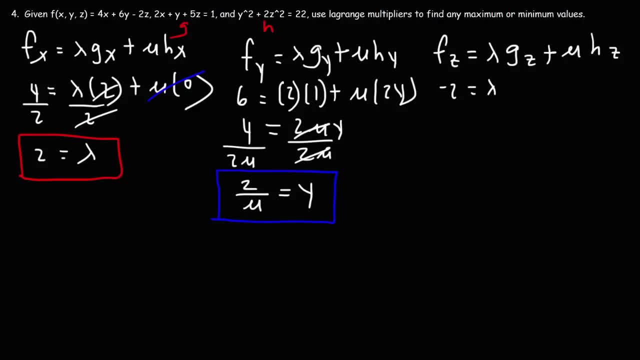 the derivative of 5z is 5.. Let's replace lambda with 2.. So this is going to be 2 times 5, plus u and then hz. The derivative of 2z squared is going to be 4z. 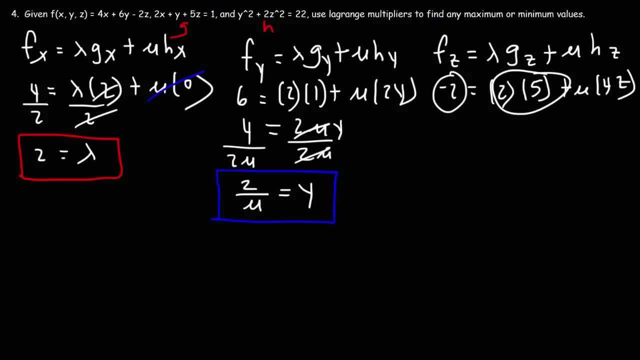 So we have negative 2.. 2 times 5 is 10.. Subtracting both sides by 10, it's going to be negative 2 minus 10, which is negative 12.. So we're going to try to isolate z. 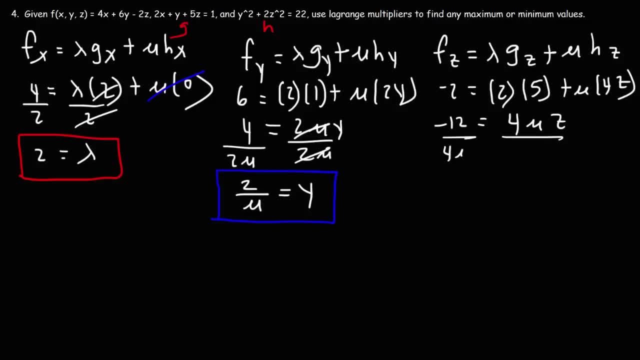 So we're going to divide both sides by 4u Negative 12 divided by 4 is negative 3.. So we have negative 3 over u is equal to z, And now let's save this expression as well. So notice that we have an equation in terms of. 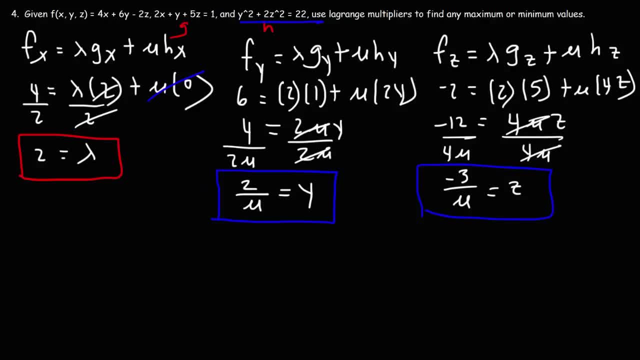 y and z. So what we're going to do is plug in or replace y with 2 over u and then replace z with negative 3 over u. So we're going to get 2 over u squared and then plus 2z squared. 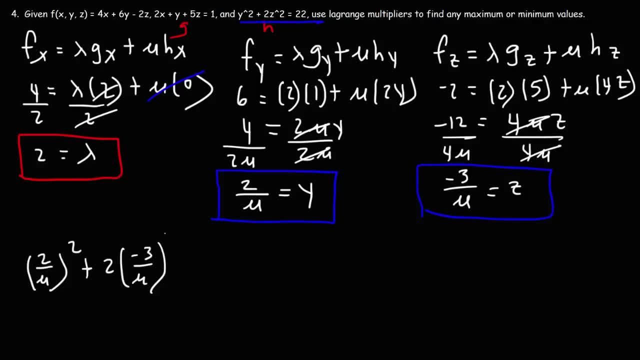 or 2 times negative, 3 over u squared, And that's going to equal 22.. So 2 squared is 4.. 3 squared is 9.. 9 times 2 is 18.. So that's going to be 18 over u squared. 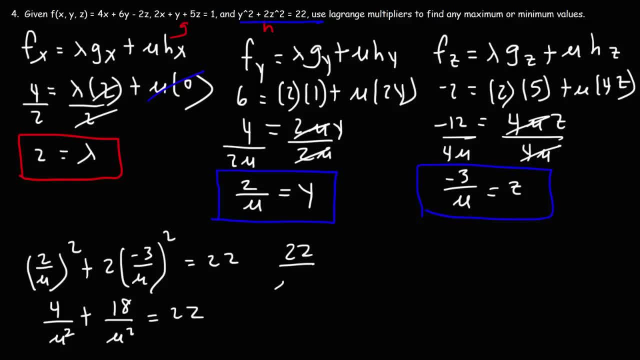 4 plus 18 is 22.. So we have 22 over u squared, which equals 22.. So this means that u squared is 1.. And if u squared is 1, taking the square root of both sides, we can see that u is plus or minus 1.. 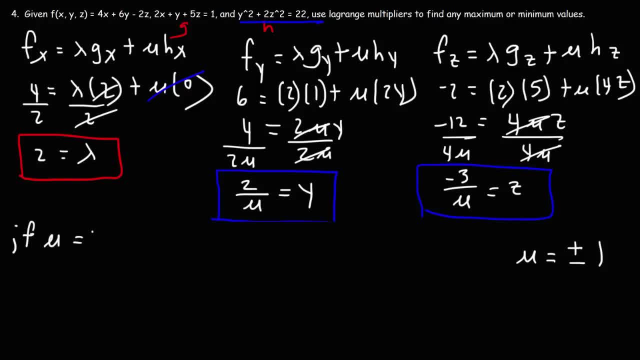 Now let's start with the situation if u is equal to 1.. So, plugging that into this expression, y is going to be 2 over u or 2 divided by 1.. So y is 2.. z is going to be negative: 3 over 1,. 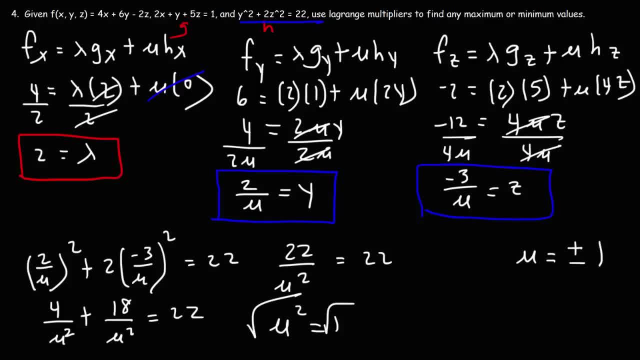 u is plus or minus 1.. Now let's start with the situation if u is equal to 1.. So, plugging that into this expression, y is going to be 2 over u, or 2 divided by 1, so y. 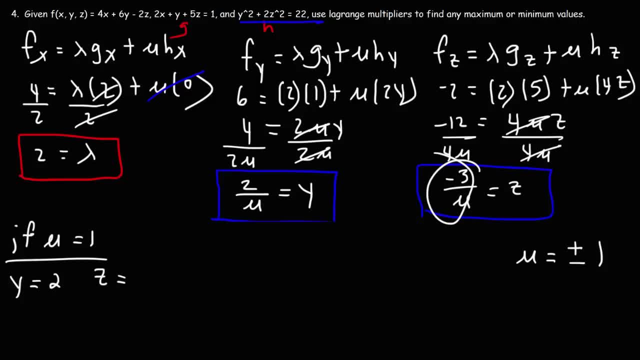 is 2.. z is going to be negative 3 over 1, which makes z negative 3.. Now we need to calculate x, and the best way to do that is to use the g-constraint equation, because it has x, y and 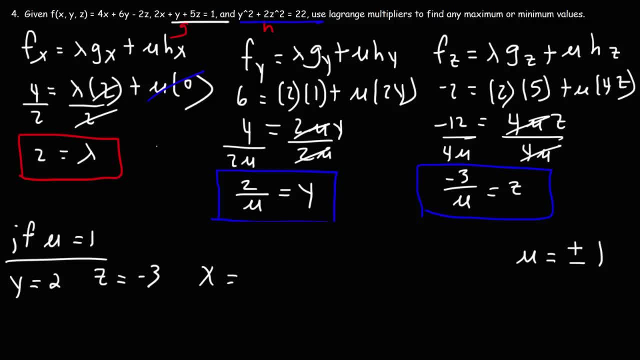 z in it. So let's plug in y and z and let's solve for x. So it's going to be 2x plus y. y is 2 plus 5z, or 5 times negative 3, which equals 1.. 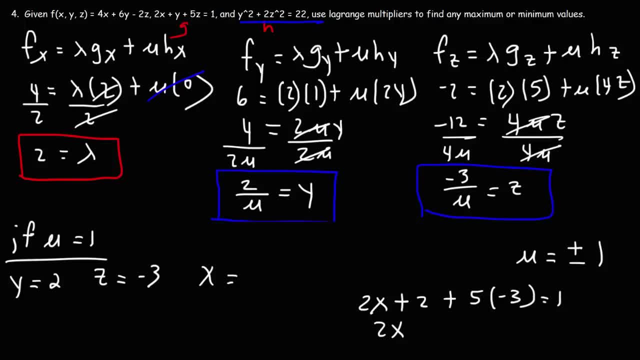 So 5 times negative, 3 is negative, 15 plus 2,, that's negative 13.. Add in 13, to both sides we have 1 plus 13,, which is 14, and x is going to be 14 divided by. 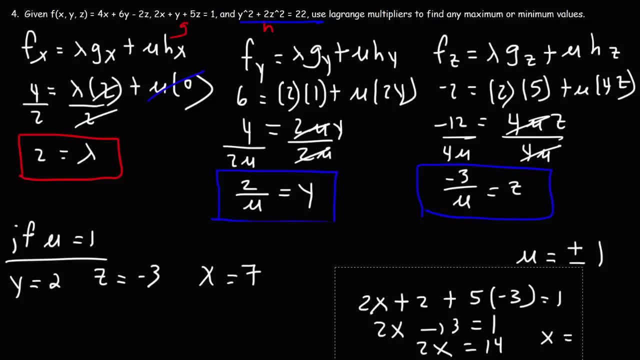 2, or 7.. So that's what we have if u is equal to 1.. Now, if u is equal to negative 1, this is going to be 2 over negative 1, so y will be negative 2.. 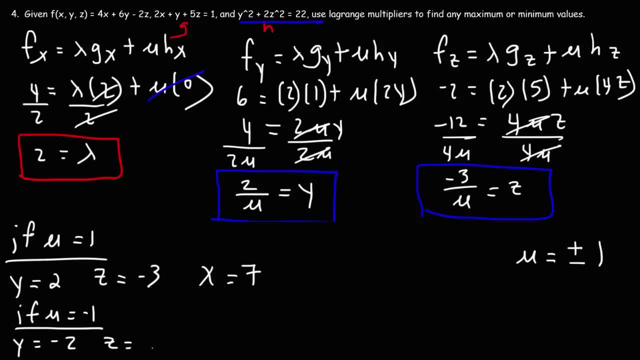 z is going to be negative 3 over negative 1, which is positive 3.. And so we need to get a new value for x in that equation. So it's 2x plus y. y is now negative 2, and then 5 times 3,. 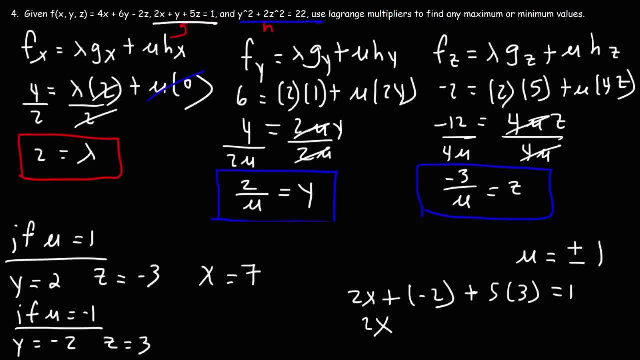 which equals 1.. So 5 times 3 is 15 plus negative 2,, that's positive 13.. Subtracting both sides by 13,, we have 1 minus 13,, which is negative 12.. Negative 12 divided by 2 is: 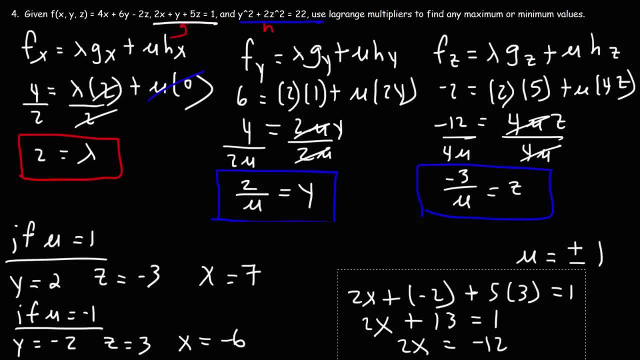 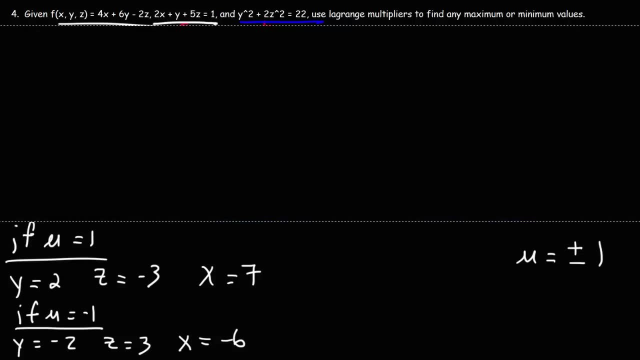 negative 6. So we get a significantly different x value in that case. So now we're going to evaluate the function at that point. So let's get rid of this. So let's evaluate f when x is 7, when y. 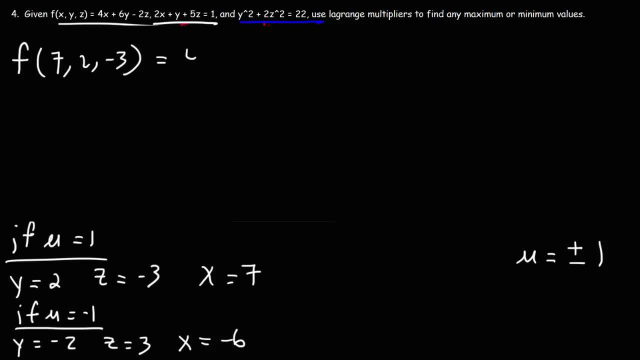 is 2, and when z is negative 3.. So it's 4x or 4 times 7, plus 6y or 6 times 2, minus 2z or 2 times negative 3.. 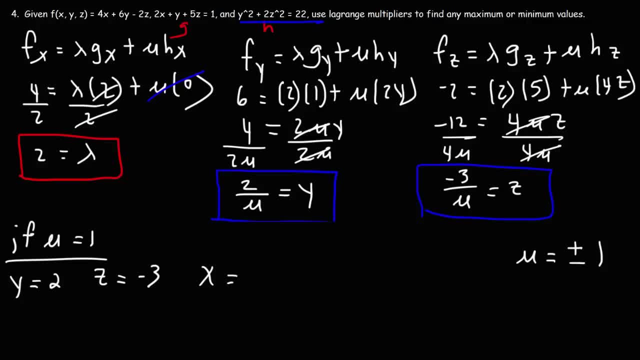 which makes z negative 3. Now we need to calculate x, And the best way to do that is to use the g-constraint equation, because it has x, y and z in it, So let's plug in y and z. 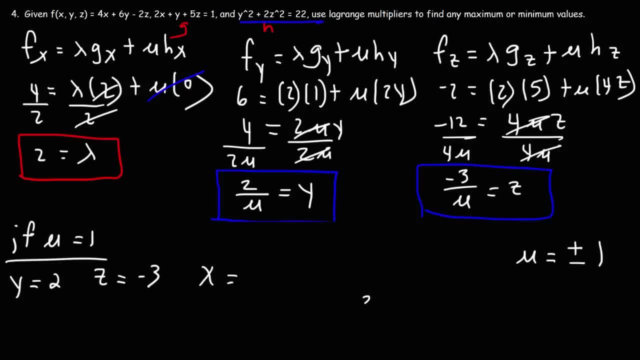 and let's solve for x. So it's going to be 2x plus y. y is 2 plus 5z, or 5 times negative 3, which equals 1.. So 5 times negative 3 is negative 15 plus 2.. 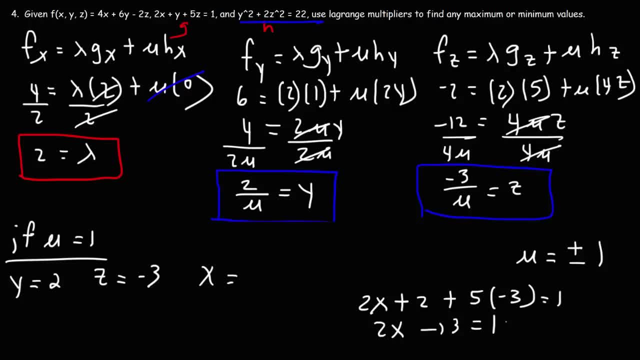 That's negative 13.. Adding 13 to both sides, we have 1 plus 13,, which is 14.. And x is going to be 14 divided by 2, or 7.. So that's what we have if u is equal to 1.. 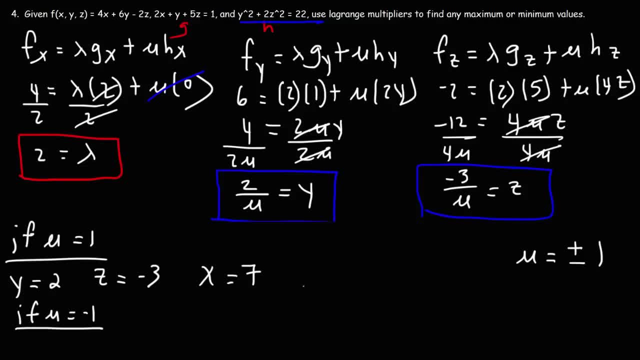 Now, if u is equal to negative 1,, this is going to be 2 over negative 1, so y will be negative 2.. z is going to be negative 3 over negative 1,, which is positive 3. And so we need to get a new value for x in that equation. 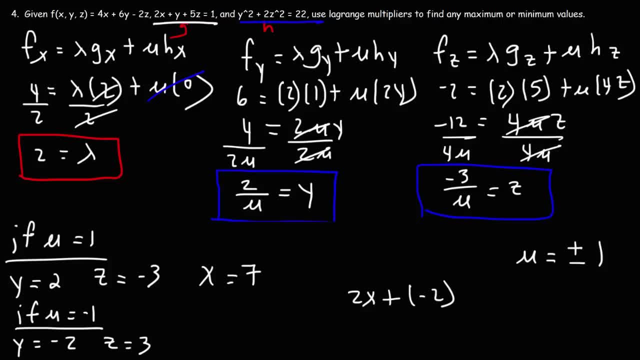 So it's 2x plus y. y is now negative 2. And then 5 times 3, which equals 1.. So 5 times 3 is 15 plus negative 2.. That's positive 13.. Subtracting both sides by 13,. 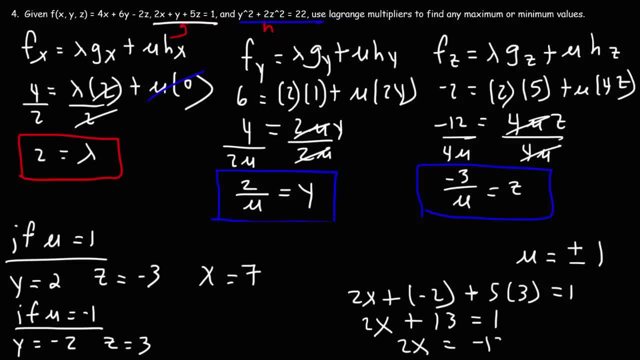 we have 1, minus 13,, which is negative 12. Negative 12 divided by 2 is negative 6. So we get a significantly different x value in that case. So now we're going to evaluate the function at that point. 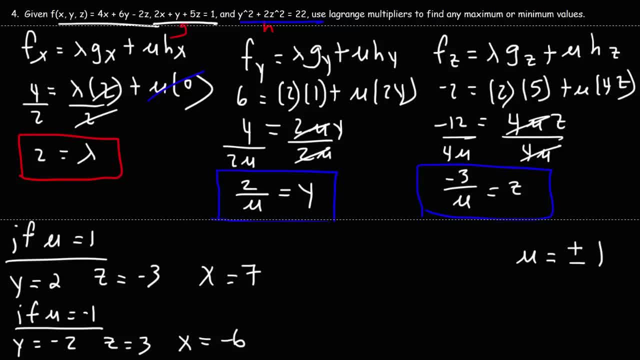 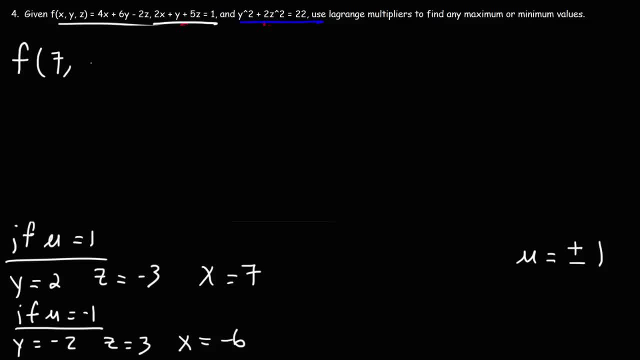 So let's get rid of this. So let's evaluate f when x is 7, when y is 2, and when z is negative, 3.. So it's 4x, or 4 times 7, plus 6y, or 6 times 2,. 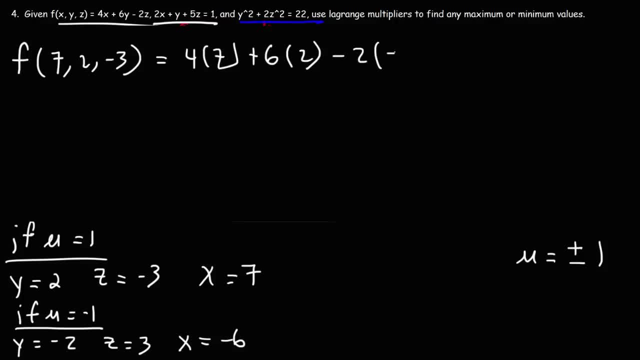 minus 2z or 2 times negative 3.. So 4 times 7 is 28.. 6 times 2 is 12.. Negative 2 times negative, 3 is 6.. 28 plus 12 is 40, plus 6.. 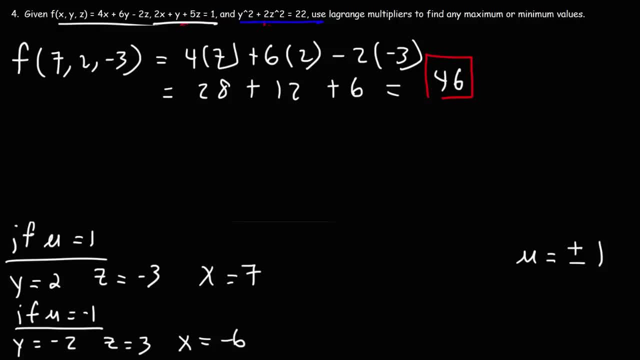 So that gives us a function value of 46.. Now let's evaluate the function at the other point: When x is negative 6, when y is negative 2, and when z is 3.. So it's going to be 4 times negative 6,.